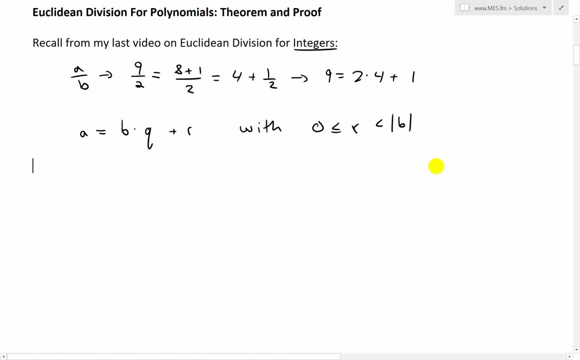 Or in other words, it's just a fraction of 2 like that, which is the remainder here Divided by 2.. Divided by the divisor, and there's the remainder R, And we can just circle this out right here. So this is what we get when we divide it. 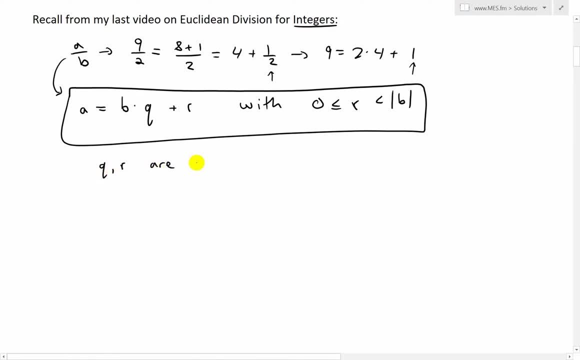 And this is again. Q and R are unique integers, as I explained in my earlier video, So make sure to watch that. I'll put that in a link in the description below. So these are unique integers. And also we have: B is not equal to 0, so we don't have A divided by 0, which is undefined, like here. 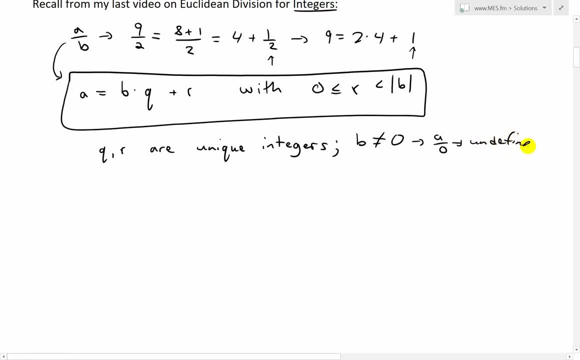 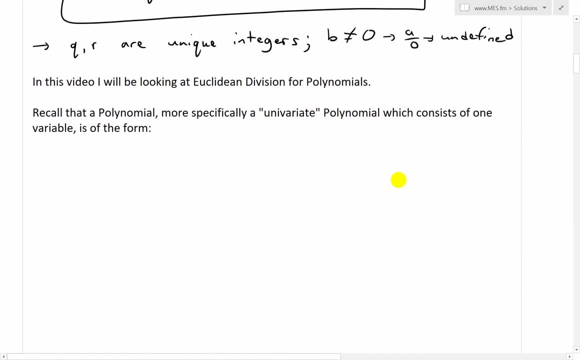 Undefined, Yeah. so now that I've gone over the recap of it, just to show you how it's pretty much very similar to the polynomials one. So now in this video I'll be looking at Euclidean division for polynomials as opposed to just integers. 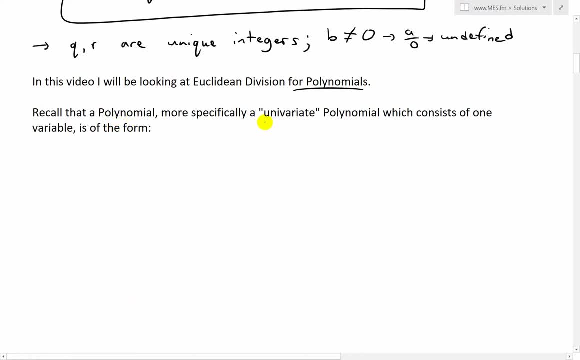 And now recall that a polynomial, or more specifically, a univariant polynomial which consists of just one variable, is of the form. And just to get a recap on polynomials, this is going to be of the form P of X, like this: 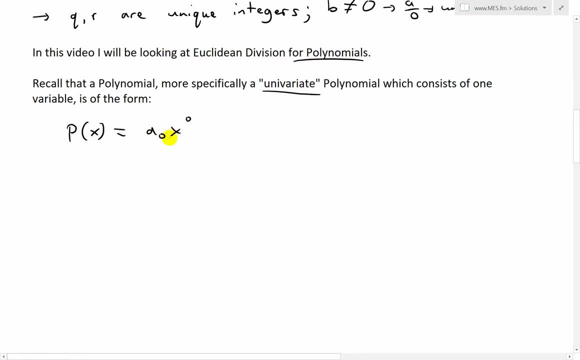 And this equals to A0, X0.. And this is just a coefficient or a constant, And this is X power of 0.. In that case, that's just 1.. Plus A1, X1.. Plus A2, X2.. 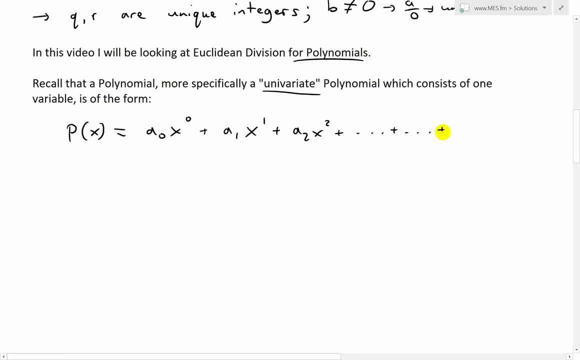 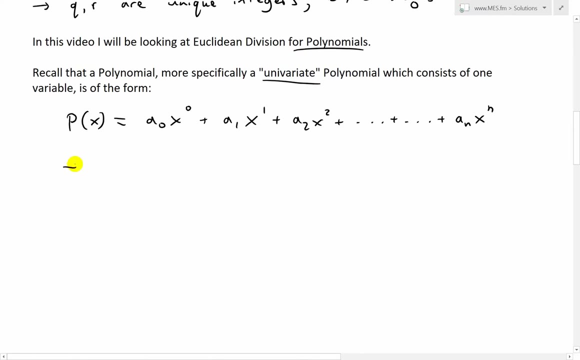 And plus keeps going on and on until finally we have AN XN. Yeah, so this is a polynomial of one variable, or a univariant, or a single variable, A single variable polynomial, and I'll write where. so, where we have the values A, I'll write AI, indicating it could be any one of these: 0, all the way to N. 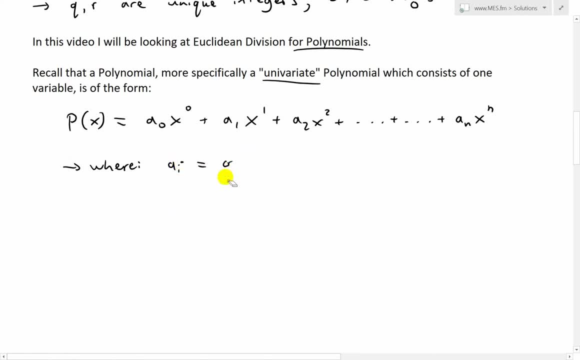 So AI, this is just a constant right here, these are just constants like that, or constants. And we also have XI, X to the power of I, where we have basically, I is equal to positive Integers, like this positive integer, integers over here. 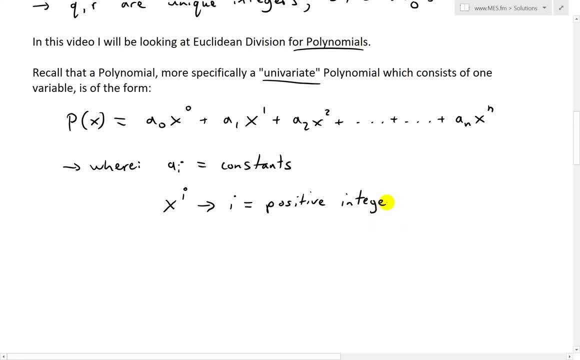 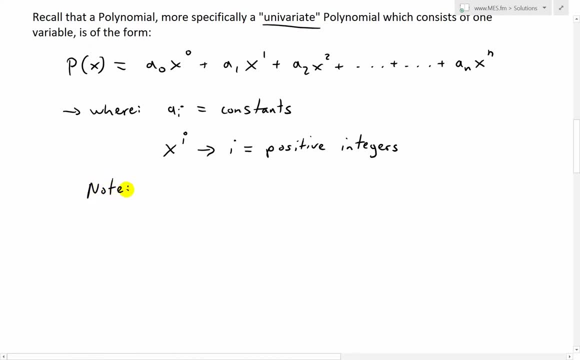 So 0,, 1,, 2,, 3,, all the way to there. so it's positive integers, Although if it's a negative one, we don't get a polynomial. And also now, what I'm going to do is note, for the cases of this video we're going to use, I'm going to call something as the leading coefficient. LC equals leading coefficient, like this coefficient. 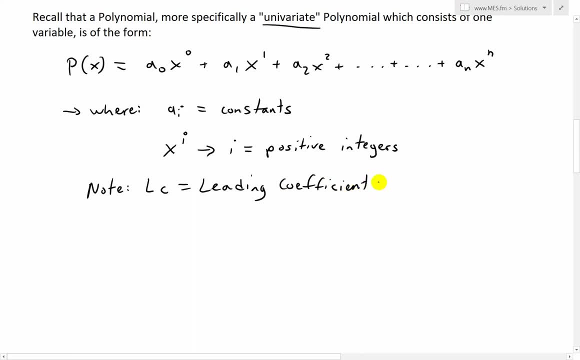 Coefficient- And I'm going to define this as basically AN there- which is equal to the coefficient of the highest degree variable, like that, or the highest degree, yeah, yeah, the highest power there- X to the N which is going to be the highest one as you increase, like that. 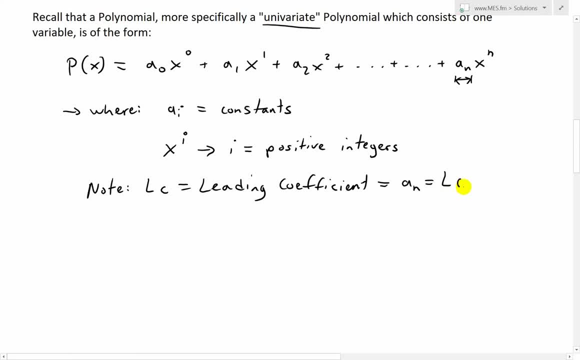 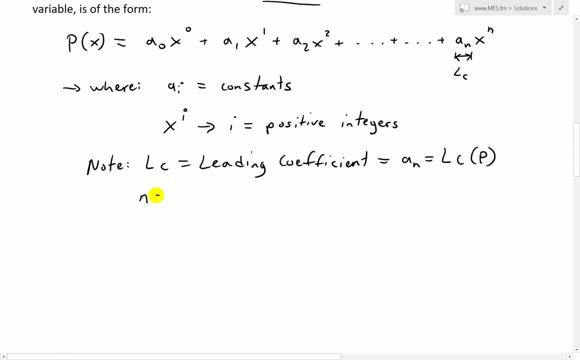 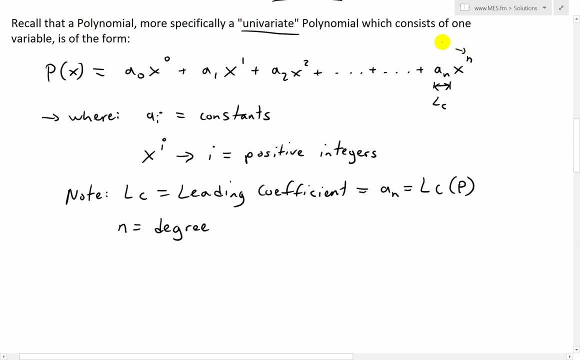 And I'll just write this as a function for this specific polynomial. so LC of P is equal to AN. this is our LC, like that, And also the degree. so I'll write N is equal to the degree of the polynomial. Yeah, so then this is the degree, like that degree, or the highest power of it. 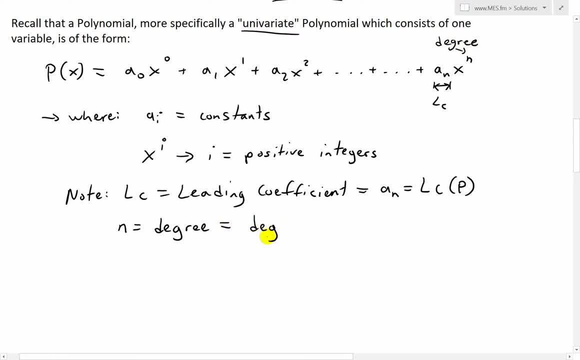 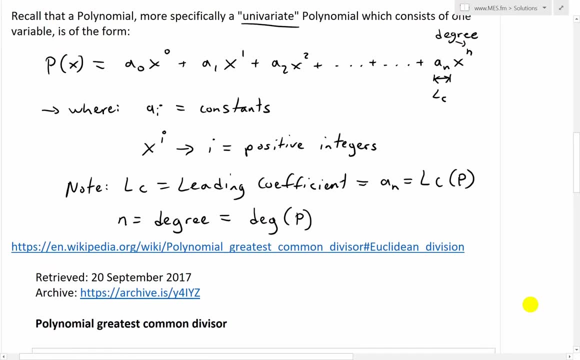 And again write this as a function. I'll write this as degree D, EG and function of the polynomial. P is equal to N, like that, Alright? so now that we have these definitions out and the polynomial, just to recap on that. 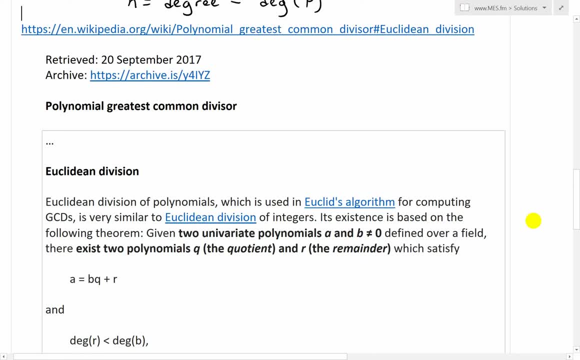 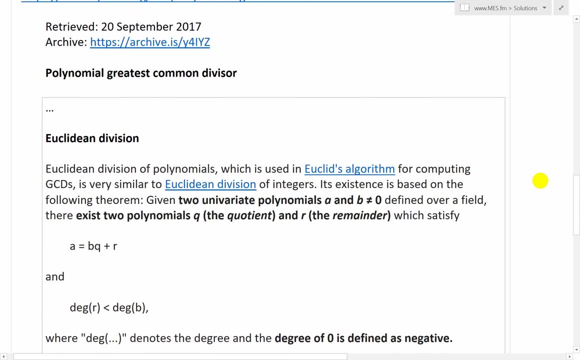 And now when we go into the Wikipedia's one as a definition and the algorithm that we're expected to prove, And it goes over the Euclidean division polynomial, So let's just go over it and then I'll go over the derivation and proof. 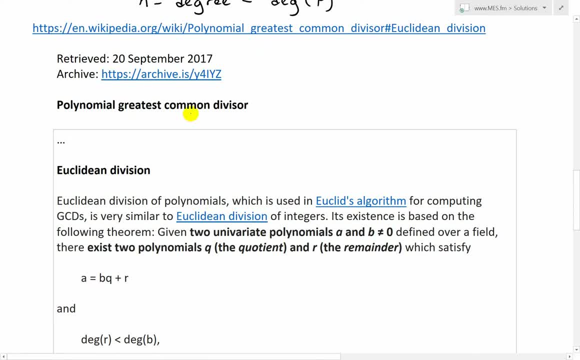 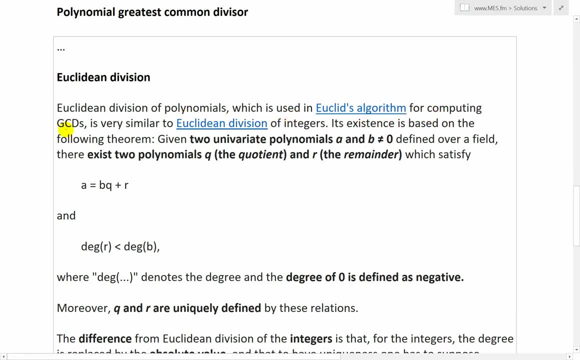 So basically, if Wikipedia has polynomial greatest common divisor in the subsection of, that has the Euclidean division for polynomials, which is used in Euclid's algorithm for computing GCDs, its greatest common divisors. I might go over those in later videos. 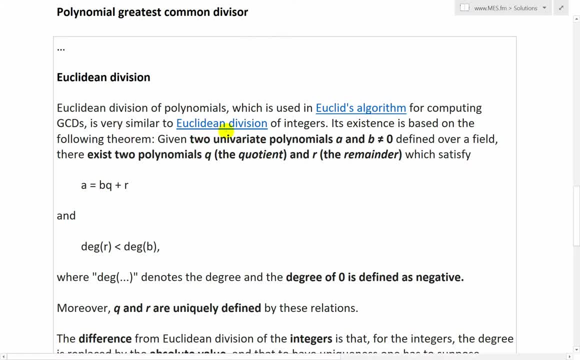 But for now that's just outside the scope of this video. So it's very similar to Euclidean division for integers. as I explained above, Its existence is based on the following theorem: Given two univariant polynomials, so polynomials with one variable. 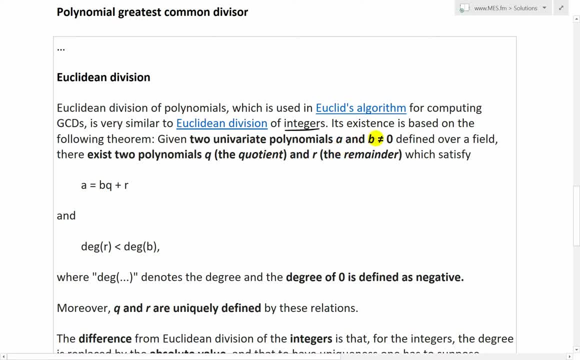 Now A and B is not equal to zero. In other words, we don't have a A over yeah, so A over B is not equal to A over zero, So we can't divide by zero like that. It'll just be undefined, as I explained above. 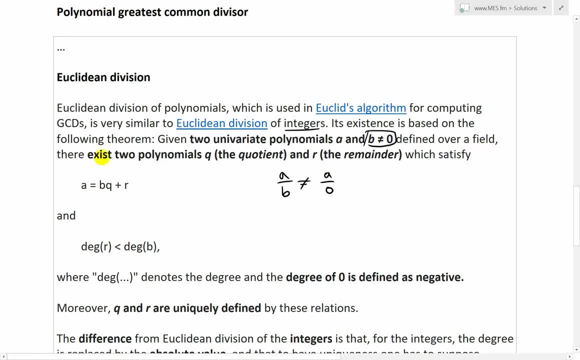 So it's defined over a field, There exists. yeah, so if we have two polynomials, A and B, there exists two polynomials: Q, the quotient and R, the remainder, Which satisfy. this formula like here and looks very similar to the integer ones. 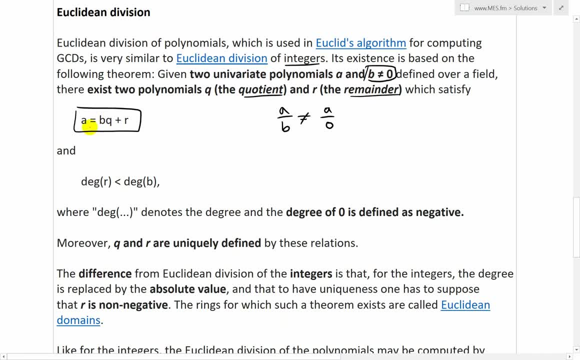 It's the exact same, but these are now polynomials. A equals B times Q plus R. A is the dividend, B is the divisor and Q is the quotient, R is the remainder, And then the degree of R is less than the degree of B. 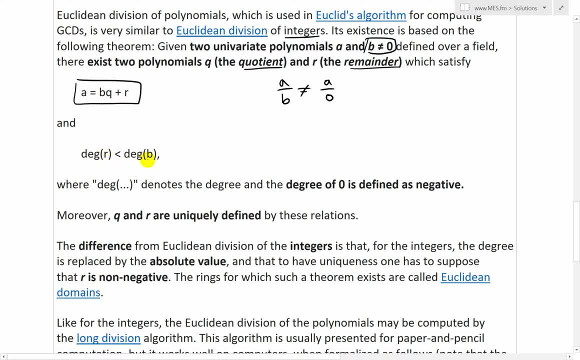 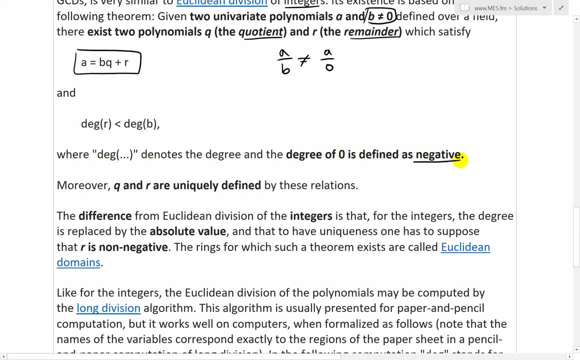 Meaning the power. the highest power of R is less than the highest power of B, Where this right here denotes the degree And the degree of zero is defined as negative. And this is actually in case- yeah, in case, and I'll explain this even further- in case, the degree of B is equal to zero. 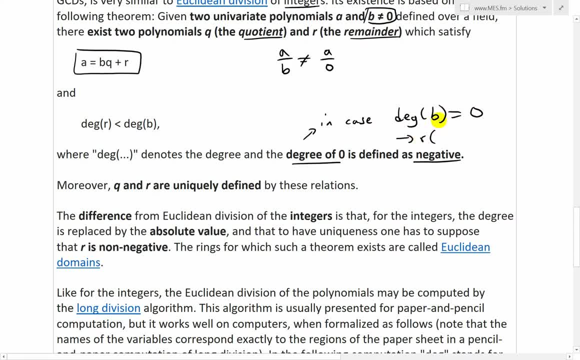 In this case, what we actually end up having is that the remainder here, in this case, yeah, the degree of zero, we're just dividing by a number, And then the degree or R of X will just equal to zero here. 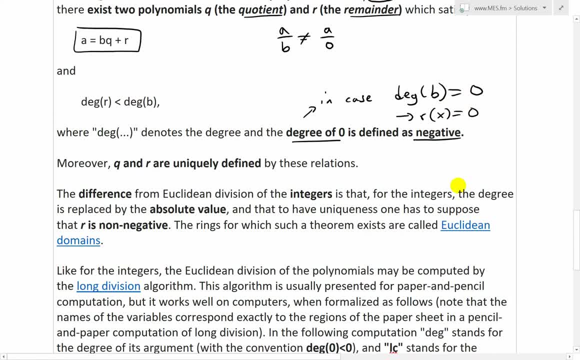 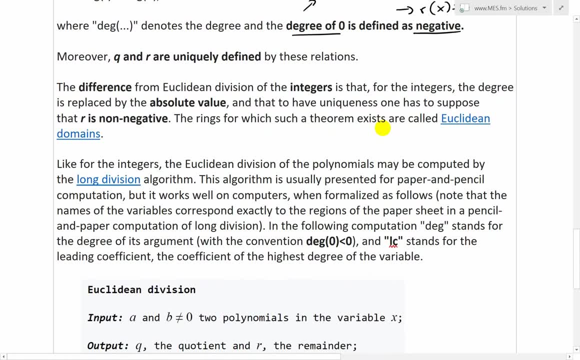 And the degree of zero is going to be defined as negative And this will make sense. So that it's negative, It's less than the degree of B, And we will go further And this will make more sense as I get in later in this video. 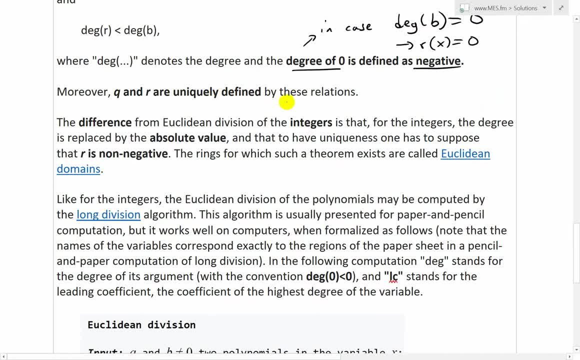 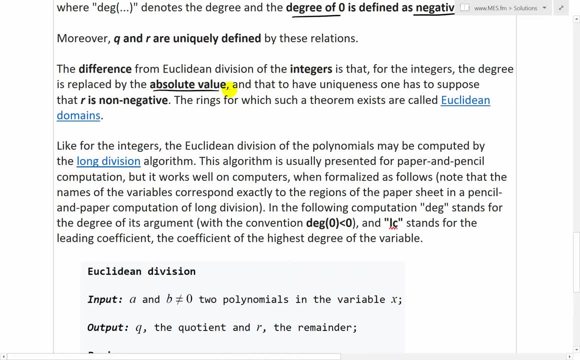 So, moreover, Q and R are uniquely defined by these relations. And now, the difference from Euclidean division of integers is that, for the integers, the degree is replaced by the absolute value of the divisor, as I explained, or B, And that, to have uniqueness, one has to suppose that R is non-negative. 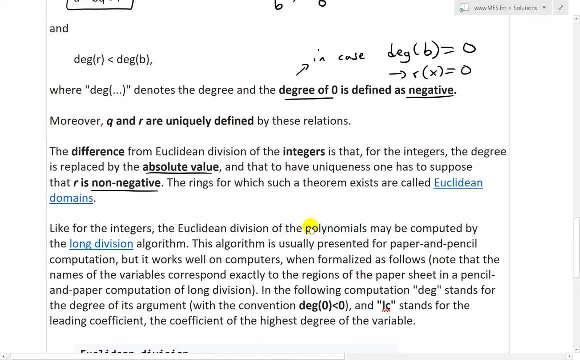 So yeah, and even in this case we're dealing with R as non-negative. Actually, I mean, that was for the other one. Yeah, for integers, you assume it's non-negative, For here all we worry about is the degree. 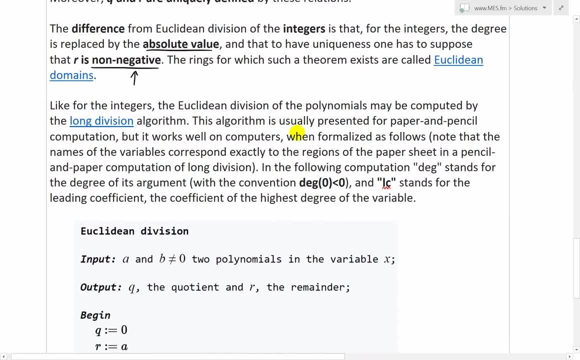 So you could have some negative values, And that doesn't matter. So that's just a difference there. So absolute value- And then we have R- is non-negative. So the rings for which such a theorem exists are called Euclidean domains, And that's outside the scope. 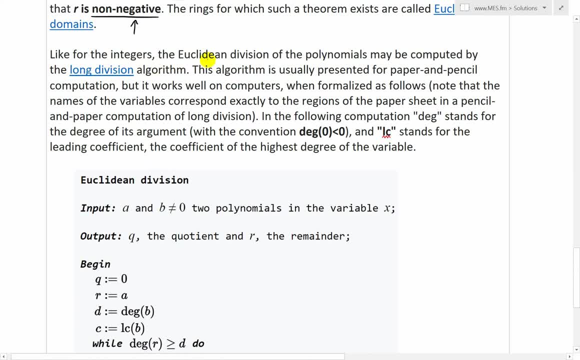 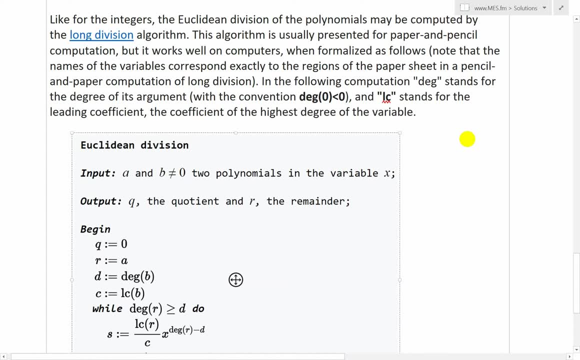 I might go into that later. So, like for the integers, the Euclidean division of the polynomials may be computed by the long division algorithm And you can learn more about long division and polynomials and integers or numbers in my earlier video. Put that in the link in the description. 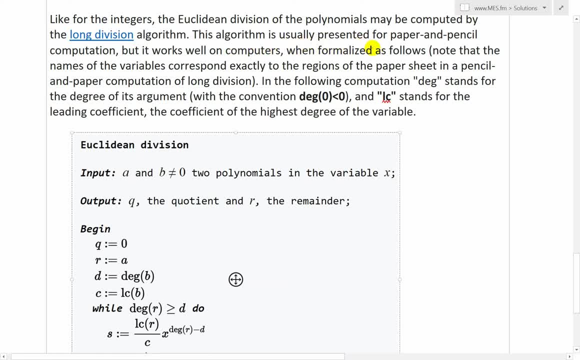 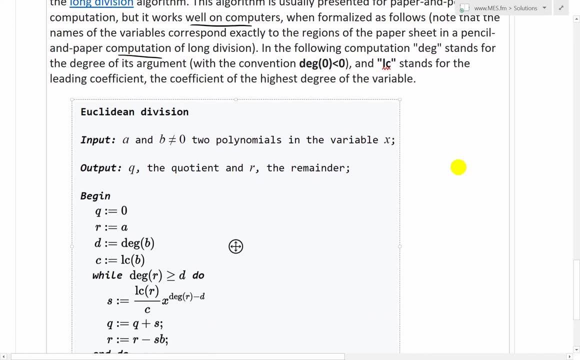 So this algorithm is usually presented for paper and pencil computation, But it works well on computers when formalized as follows. Note that the names of the variables correspond exactly to the regions of the paper sheet in a pencil and paper computation of long division. So pretty much long division. 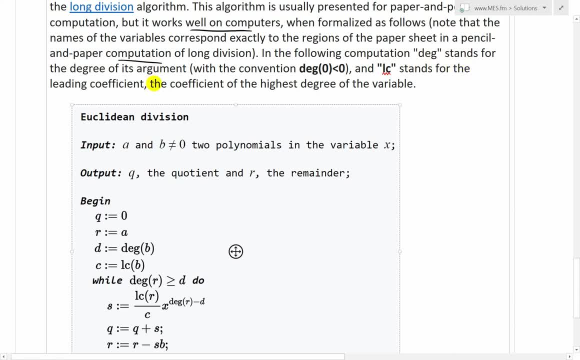 In the following computation the degree dig stands for the degree of its argument. with the convention, degree 0 is less than 0. So degree of the function 0. That is just R. X equals to 0. And again they have L, C. 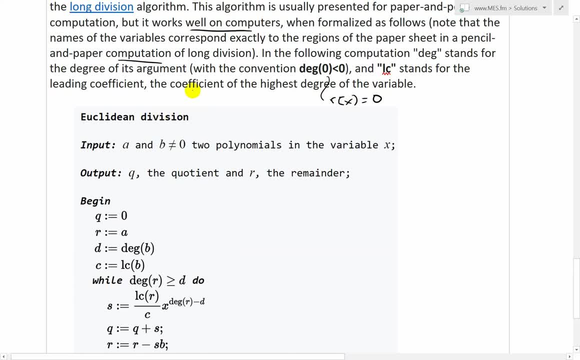 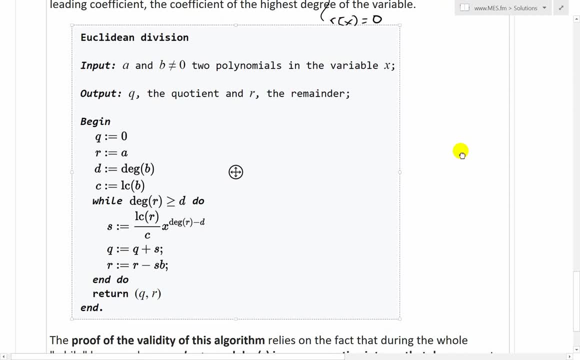 L is lowercase, It stands for the leading coefficient, as explained above, which is just the coefficient of the highest degree of the variable. And here is what they have written here And this is Euclidean division. There's that algorithm here. This is input A and B is not equal to 0.. 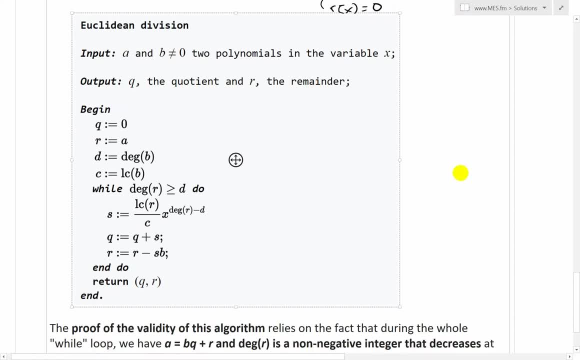 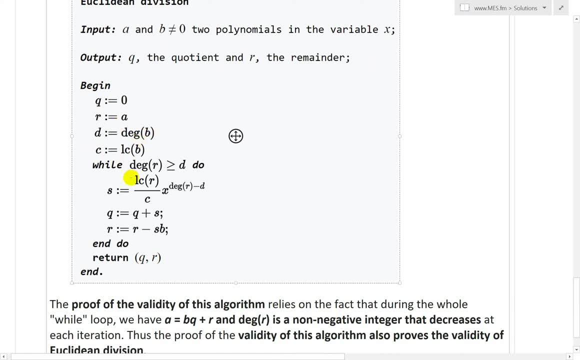 Two polynomials and a variable: X. Output Q, the quotient R, the remainder. And it has a function here. Begin: Q is 0.. R is A, Then D is degree- here You're just defining these. And then it says: while the degree of R is greater than degree of B, like here: 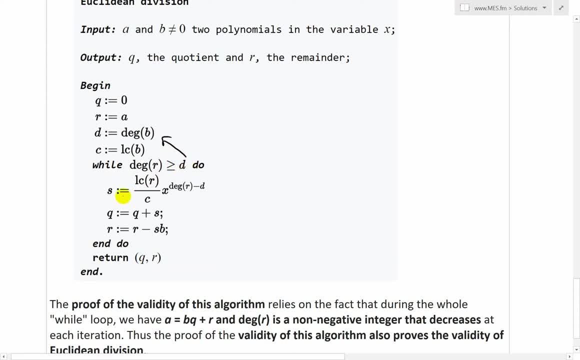 This is while this is true, so it's not less than it Do this, Then it has an S value, And I'll explain why they have it like this. They've chosen the leading coefficient of R divided by leading coefficient of C. 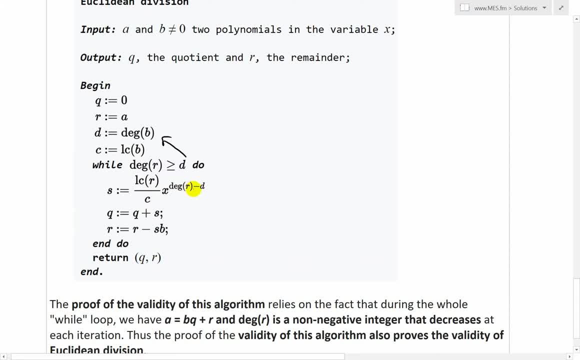 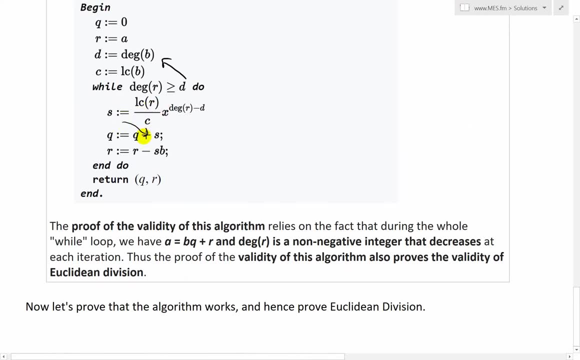 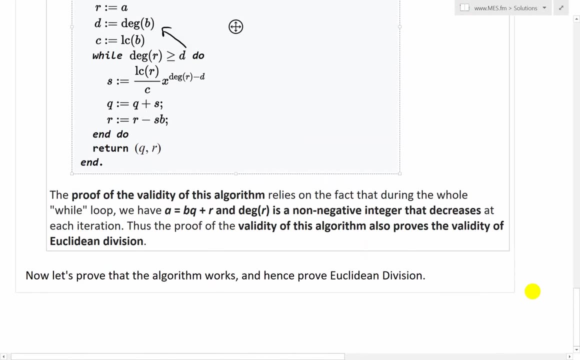 I know leading coefficient of B over there times by X, Then degree of R minus degree of B over there. Then they've added S to the Q And it keeps going on, It keeps repeating, And I'll explain this in a step-by-step method just to illustrate it, prove it and show that it works. 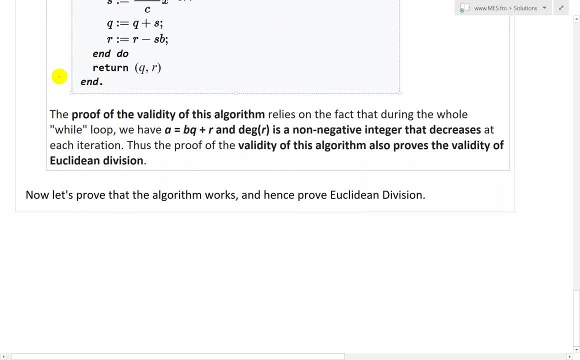 And explain what it does in a bit, But first let's read further. So the proof of the validity of this algorithm relies on the fact that during the whole while loop we have A equals BQ plus R And degrees. R is a non-negative integer that decreases. 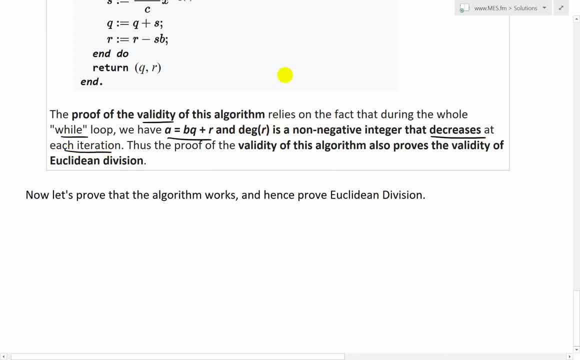 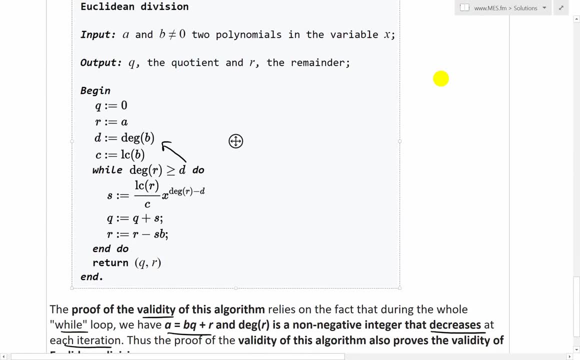 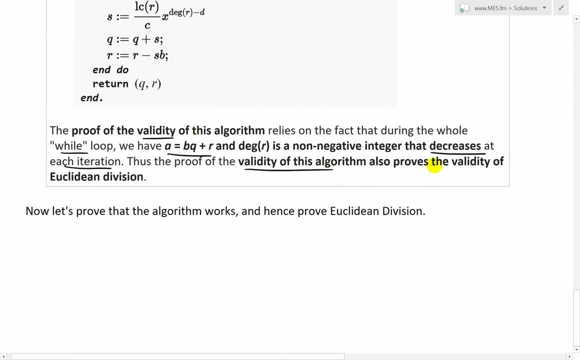 So the degree of it keeps decreasing at each iteration And then you basically stop once you have a degree of R is less than the degree of B, And thus proving the theorem. So that's always valid And it's just keep going. So thus, the proof of the validity of this algorithm also proves the validity of Euclidean division. 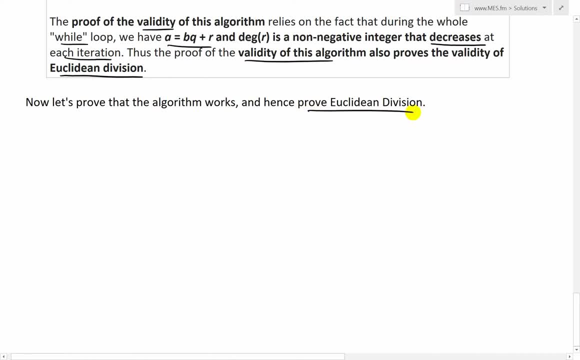 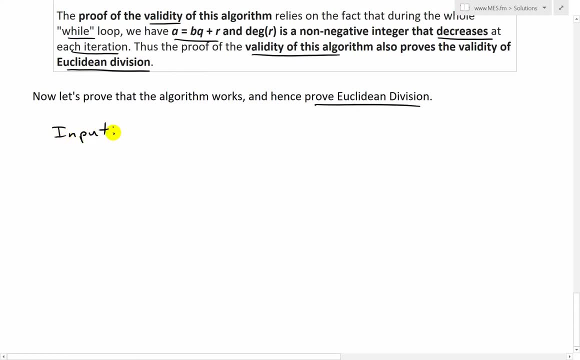 So now let's prove that this algorithm works, and hence prove Euclidean division. Yes, so to make sense of all of this, what I'll do first is: well, I'll write: the input is: So we are inputting A over B. 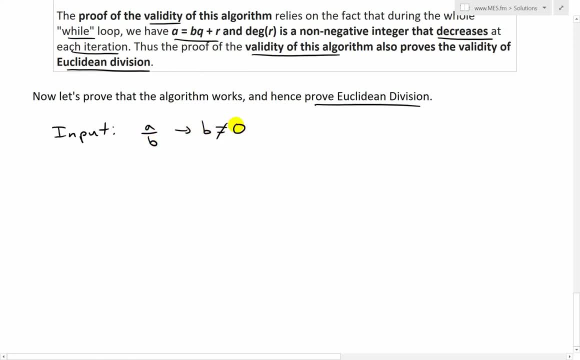 Where we have B is not equal to 0. So these are two polynomials and also both are functions of X, like here of X. So these are both polynomials of X. I'll put this in bracket: polynomials like that. 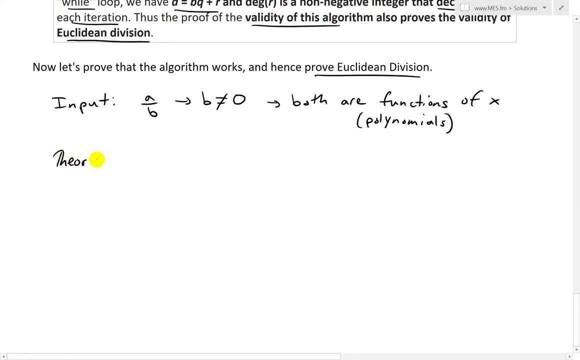 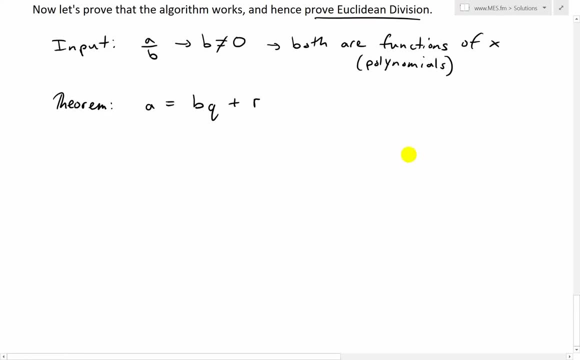 And now what I'll do is write the theorem out. So the theorem is just the Euclidean division: A equals to B, Q plus R. And now where each of these polynomials, we're going to write these as, And I'll write where these are all polynomials: 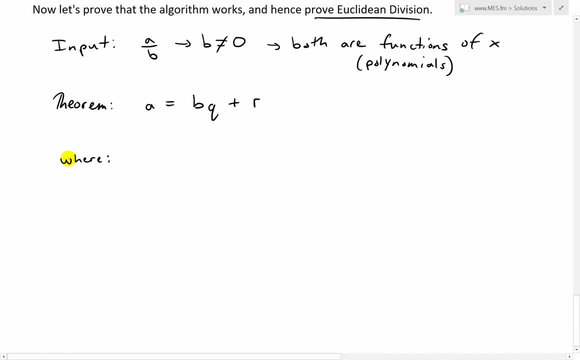 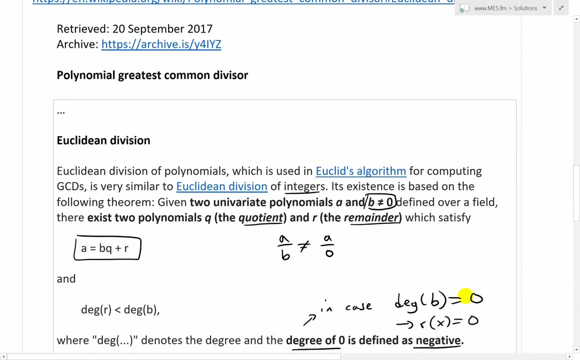 And now what I'll do is I'll use the leading coefficient method And I'll write this as: where A of X is a polynomial, And I'll write this out. So, if we go back to the polynomial, how the form of it? like this: 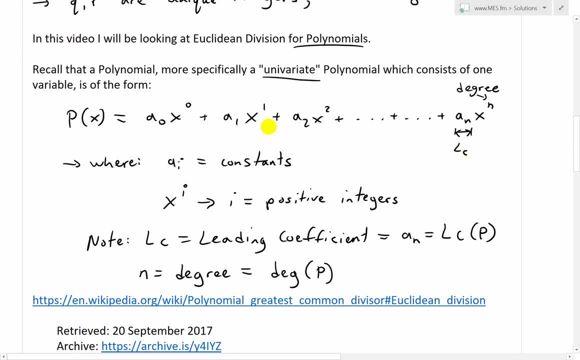 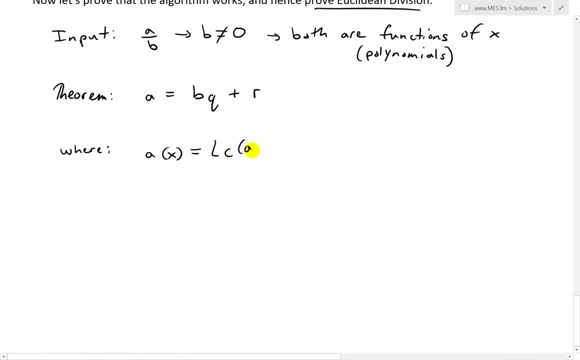 What I'm going to do is I'm going to write this L of C in front And then these ones. they don't matter much And I'll explain why. So I'll just write this as the leading coefficient of A, times it by X to the power of the degree. 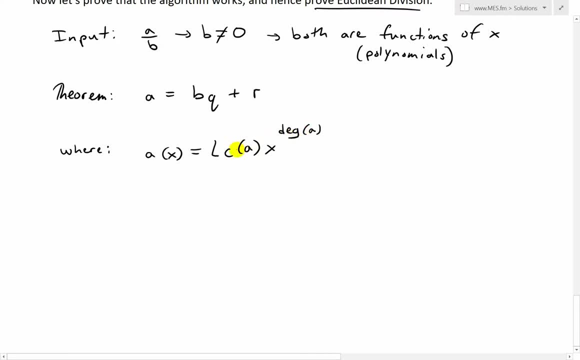 of A like this. Remember, that's just N. This is just AN Like this. This is just AN, This is just N. Yeah, so that's just N like that. And then I'm going to do this plus: dot, dot, dot. 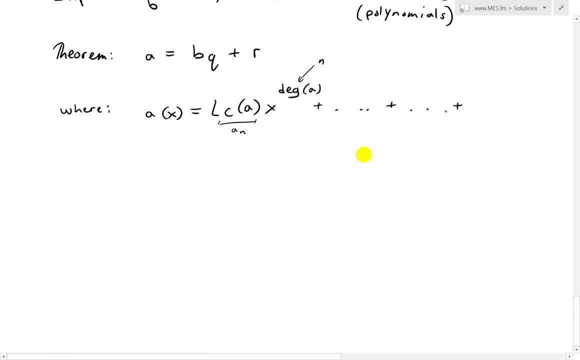 It's just the rest of the entire one. It could be A0,, A1, and so on, But I just move this in front. And then same with the B of X, the divisor. This equals to LC of B. the leading coefficient of it times X to the degree of B. 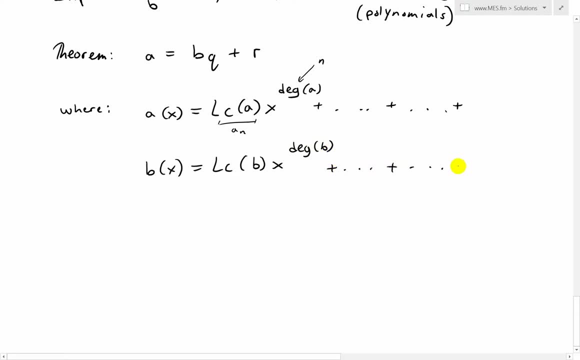 And then, likewise, we're going to have dot dot dot plus dot dot dot and so on, And then now what we have here is C of not C, this is Q. So the quotient Q is also going to be written like it, as the leading coefficient, as X. 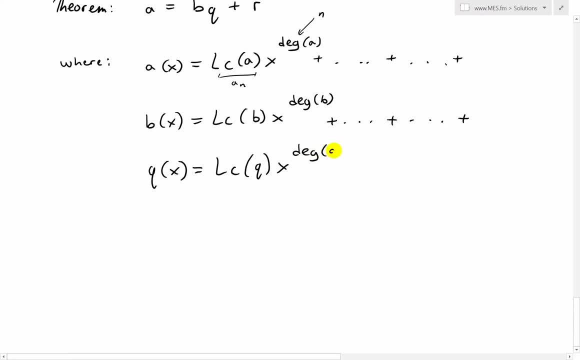 to the degree of Q or the highest power, like this, and then plus dot, dot, dot, dot dot dot, And then we're going to have R1, the remainder, which is going to be in a similar way: L of C of R, X, degree of R plus dot dot dot, plus dot dot dot, and so on. 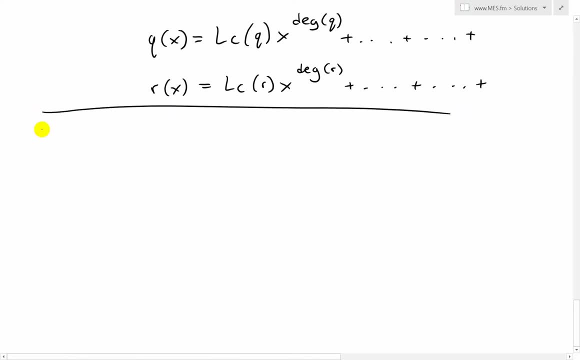 And now, before I get to the algorithm. but first let's just look at an example of long division to illustrate it, and then later, once I prove the algorithm, I will be basically revisiting the same example and do it using the long division. 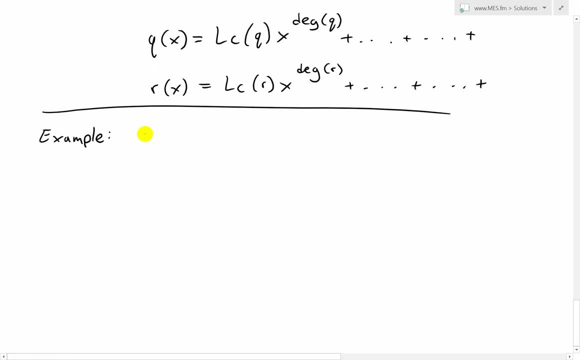 I mean the Euclidean equation. I mean the Euclidean equation, I mean the Euclidean division algorithm. So for long division, let's say we had a function X plus 3 squared as polynomial divided, by now we have 2X plus 2.. 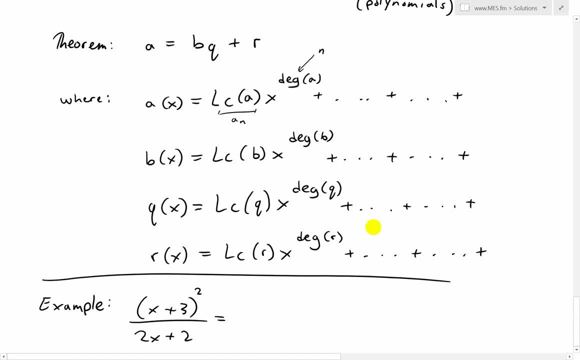 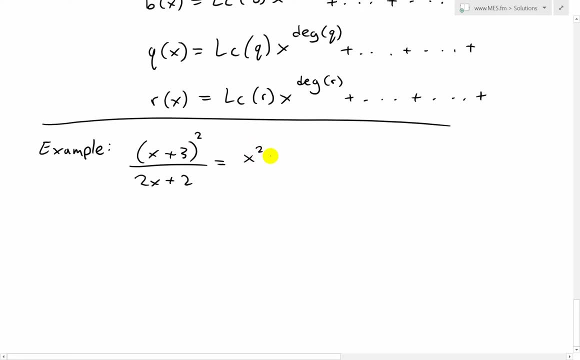 So this one first. we could just expand this. write this in the form we are used, to just expand it as the P of X form, as above. So to multiply this out, this will be: X times X is X squared plus X times 3 is 3X, and. 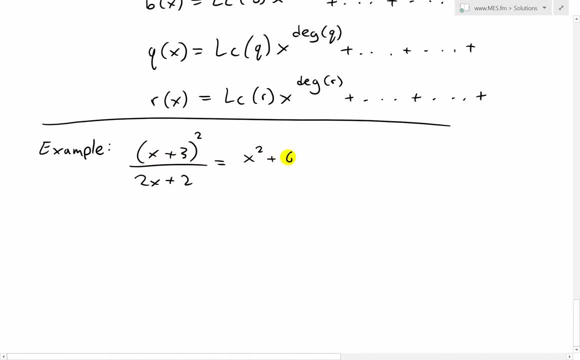 then plus 3 times X, that's 3X again. so we can add them up 6X. So 3 times 3 is not. it's using the FOIL method. and then the middle part is in my head. 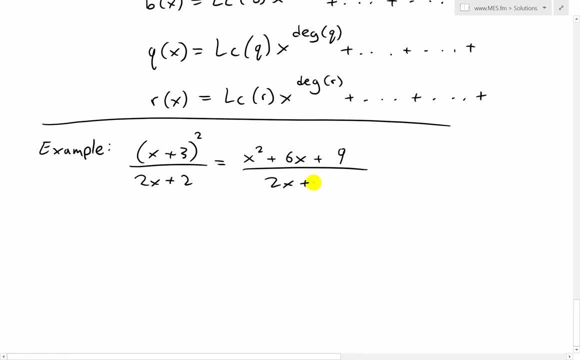 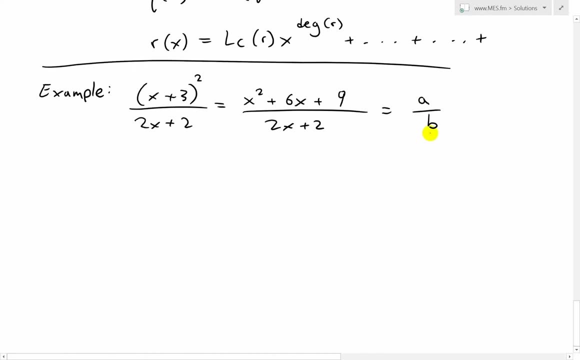 So we have like this: And then divided by 2X plus 2.. Yeah, so in other words, this is our A- let's write this as A divided by B is the polynomial, the divisor, that's the dividend. And now using long division, so long division, right here, just to illustrate it, and I'll 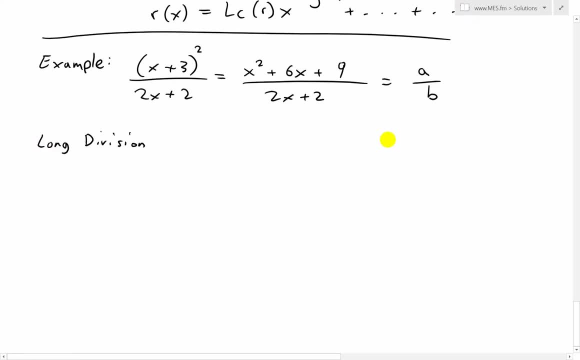 put this L, So what we end up having is a division like this: 2X plus 2, and then put this above: X squared plus 6X and then plus 9.. And you can learn more again about long division. I'll put the video link in the description. 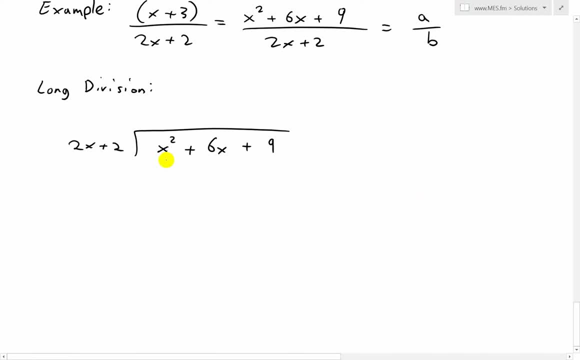 below for my earlier video. So now what we have here, what we do is remember. the method is: we need to multiply a variable here to get this 2X, and what we'll do is: well, that's just going to be, that's just. 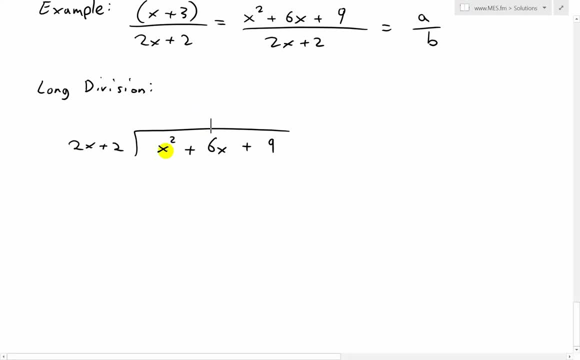 going to be X. Actually, no, the other way around. we need to get the X squared, my bad. so we need to cancel the X squared, And what we'll do is multiply this 2X by- well, 1 half X. 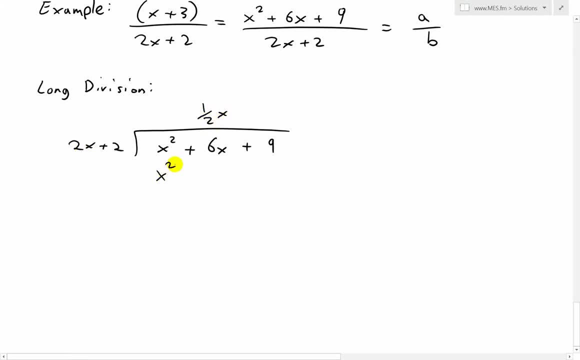 So when we do that, what we get is an X squared, and then this one. by this, the 2's cancel again. we'll just be left with plus X, like that, and then we can just subtract, And when we subtract, this cancels, and now we have this 6X minus X, that's just 5X carry. 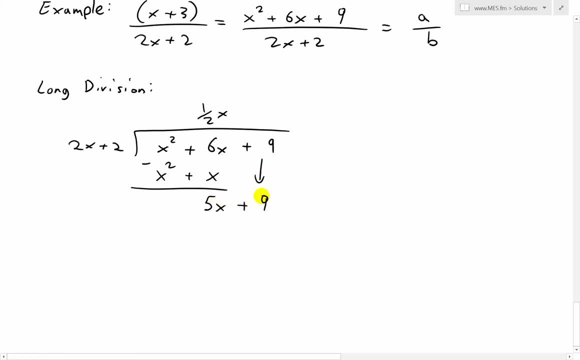 the 9 down, we have plus 9 like this: And now what we have over here, we need to get the 5X. so we multiply over here by plus 5.. 5, well over 2X, like actually. no, just leave the X out. so 5 over 2,. so 5 over 2. 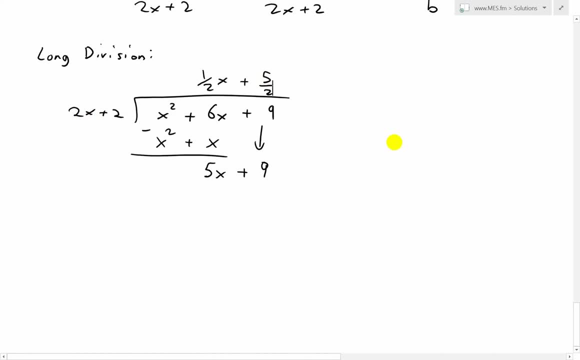 times 2X. that just becomes well the 2's cancel, that's just 5X. So we have 5X, and then over here the 2's cancel again, that's just plus 5, like that. 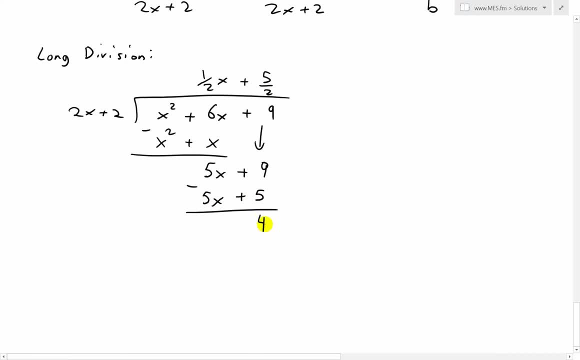 subtract. this cancels. now we have 9 minus 5 is 4, and now we can't get any further to this one. so that's the remainder. So this is R. I'll just write this as R of X. 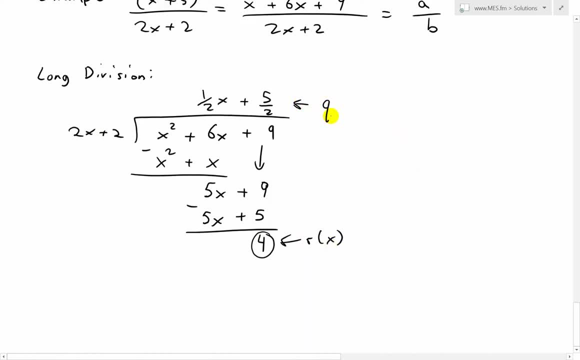 Like that. And now this whole thing on the top is the quotient Q of X. Yeah, so thus what we have. we've written in the Euclidean division form. so thus, well, before we get to that, yes, we have over there the whole thing, so let's put this over so. 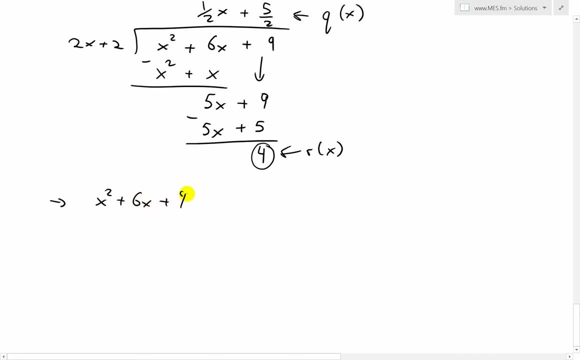 we have X squared plus 6X plus 9, I'll just write thus here. So thus, X squared plus 9, all divided by 2X plus 2, equals to the quotient 1 half X plus 5 over 2, and then plus the remainder 4,. in other words, then, when we multiply this: 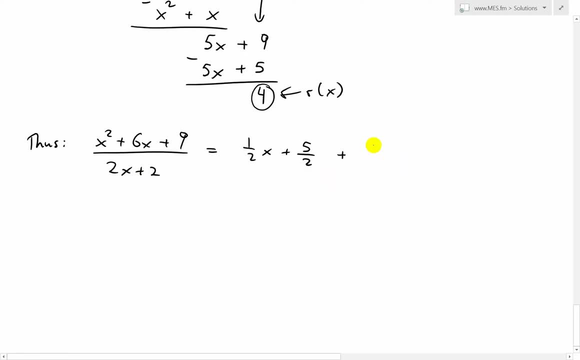 on both sides. actually, this is the fraction plus 4, and it can't divide evenly, so we just leave it out there and it's just 4 divided by 2X plus 2,. remember, that is the long division. 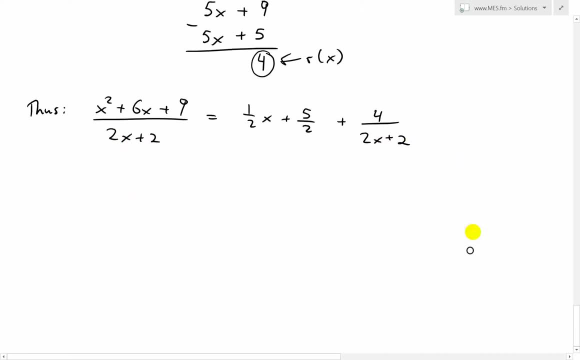 method. Now, when you multiply by 2X plus 2 on both sides, we can cancel that. what we end up getting is an X squared plus 6X plus 9, equals to- now- let's put this in front- 2X plus 2,. 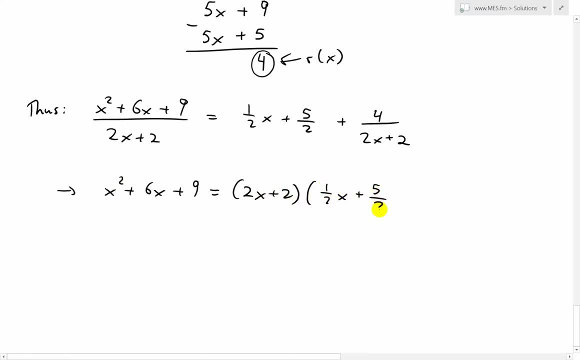 and then we have this 1 half X plus 5 over 2, and now we have plus the 4, so the 2X plus 2 cancels out like that. Yeah, so in other words, here we have our A equals to here's B, and here is the Q. 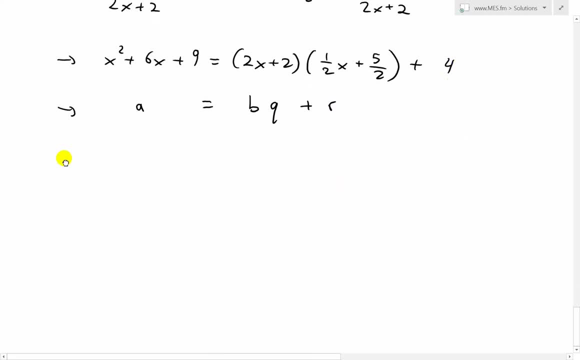 and there's the R, like that, And thus what we end up having is- I'll put this out like this: each of the functions, so A of X. to make it like the other one, A of X equals X squared plus 6X plus 9, and. 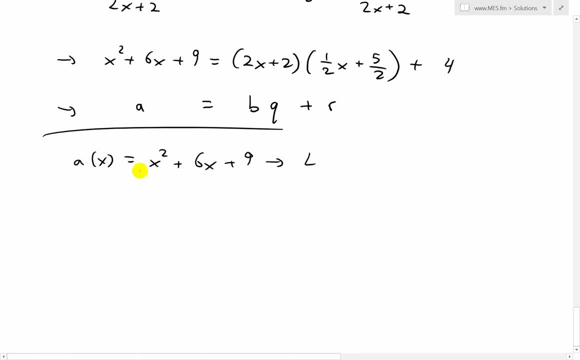 in this case we have the leading coefficient is going to be well, just 1, leading coefficient of A equals 1, and then degree here is 2, degree of A equals 2,. likewise for our B of X, that just equals to our 2X plus 2,, 2X plus 2, and then that leading coefficient of B. 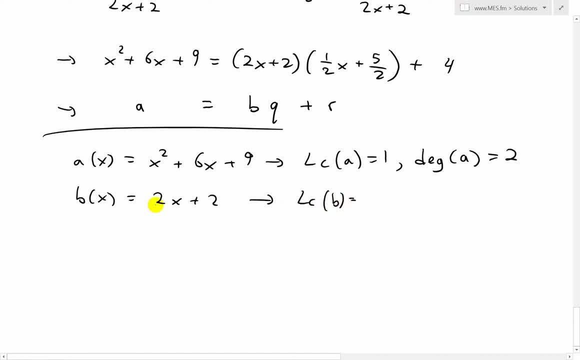 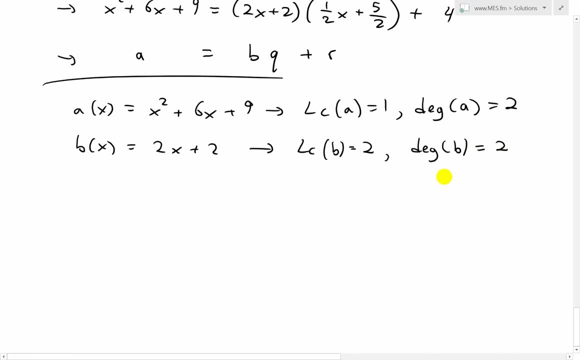 is going to be equal to 2, so that's the leading coefficient And then the degree of B. B equals to 2, like that. Yeah, I mean the degree of B is 1, because that's the power of 1 over there. likewise, 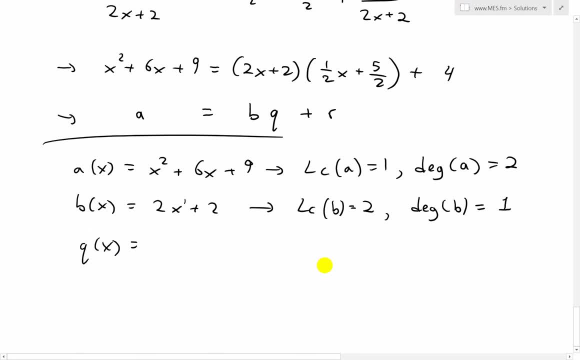 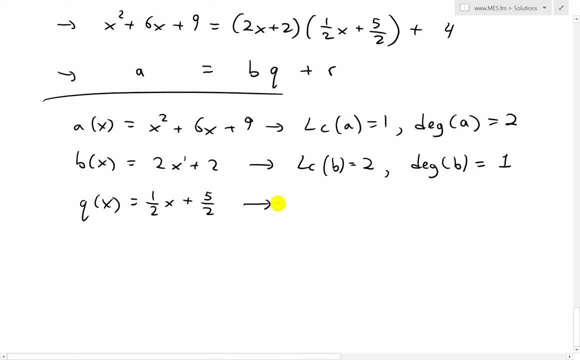 for the Q, Q of X equals to, that's 1 half X plus 5 over 2, now the degree or the leading coefficient is going to be 1 half and the degree of it is just that's going to be 1. 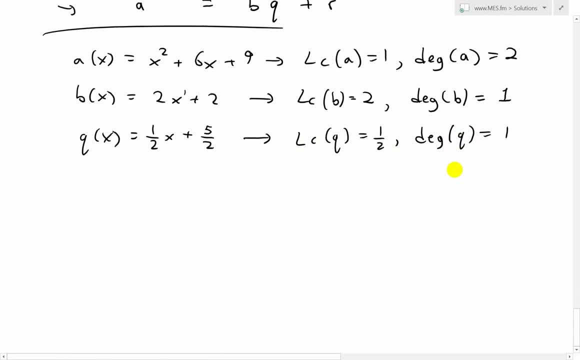 as well. again, Equals, Equals, 1.. And then, last one is: the remainder is just remainder. R of X is just equal to. yeah, the remainder is just going to be equal to 4. over there, that's just 4, so then the leading. 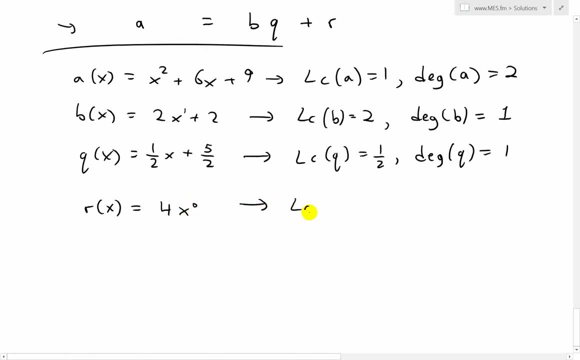 coefficient. again, you could think of it as X to the power of 0, leading coefficient is just 4, that's the highest power. there is 0, this is going to be equal to 4, and then the degree of R equals to 0. 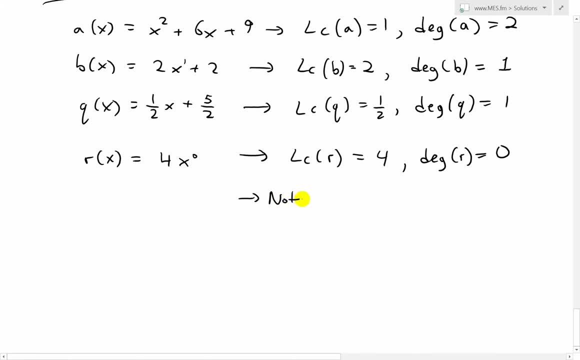 And also notice, note that the degree of R is less than the degree of B. The degree of R equals to 0,, which is less than the degree of B, which equals to 1.. So yeah, this fits our Euclidean division. 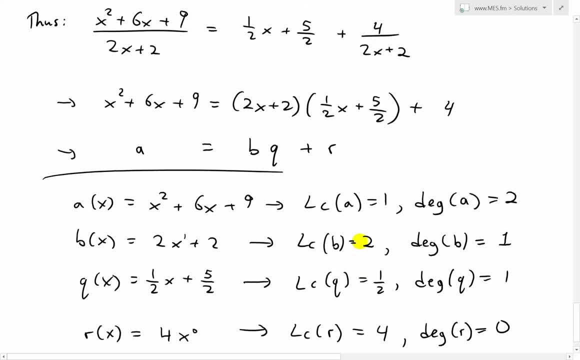 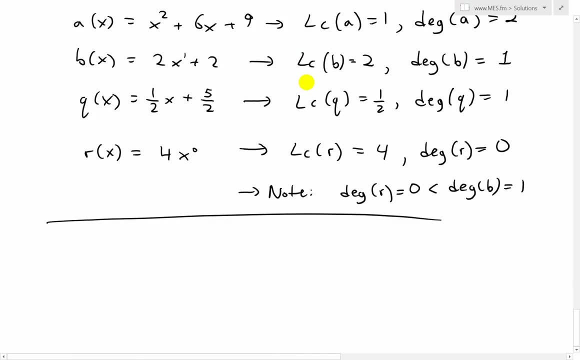 And now to prove that algorithm, just to give you an example of how to define all these terms, just to illustrate it further, and then later I'm going to show the Euclidean division, In fact same thing as the long division that I just did over here. 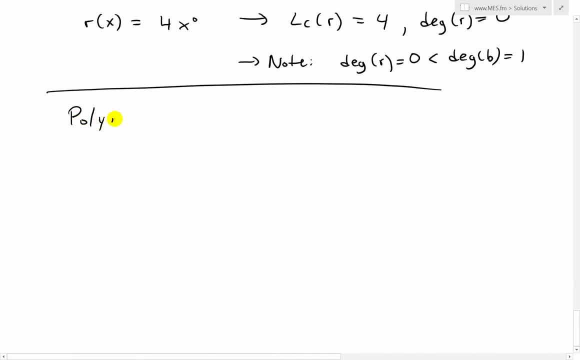 Yeah. so thus what we have is: let's just go over our polynomial long division, or polynome, yeah, polynomial, yeah, division algorithm like this, yeah, algorithm. And then this will prove the Euclidean theorem there. 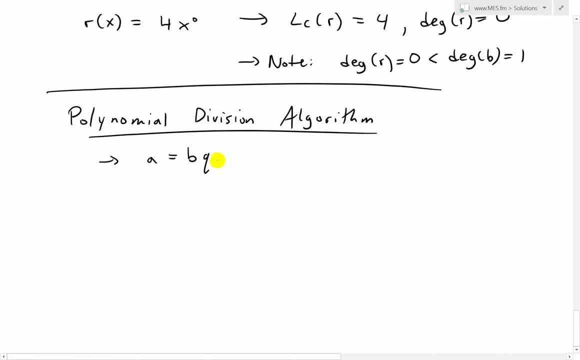 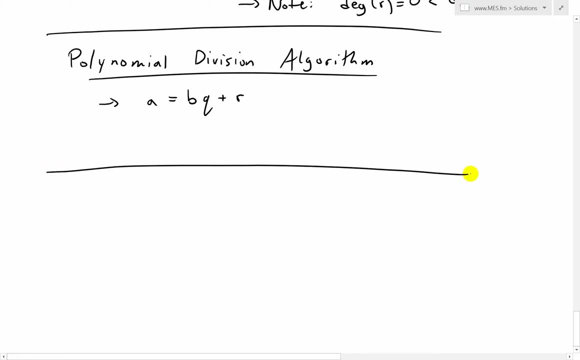 So what we have first is we always have: A equals to B, Q plus R is our theorem. we always need to have. And now what I'll do is I'll make a giant table like this and I'll write this as the first column is just going to be the row number number like that, and put it out somewhere. 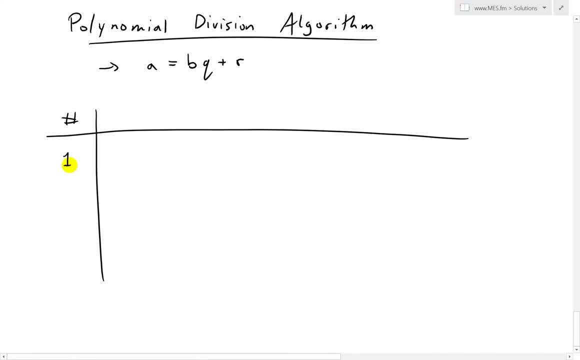 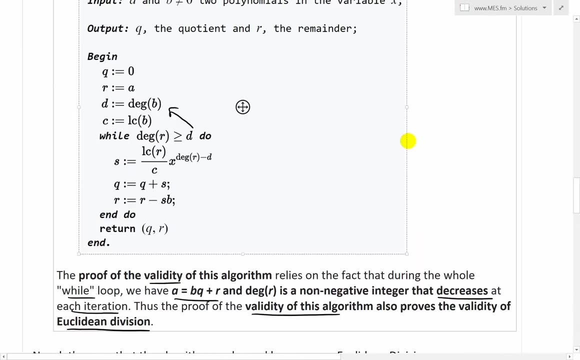 over there. I'm going to call this one 1, so row 1.. Then we have our Q values and remember as above in that giant table and I'll just be going through it. it's pretty straight forward when you go through it. 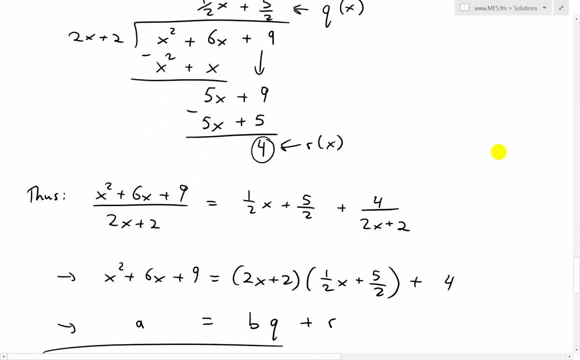 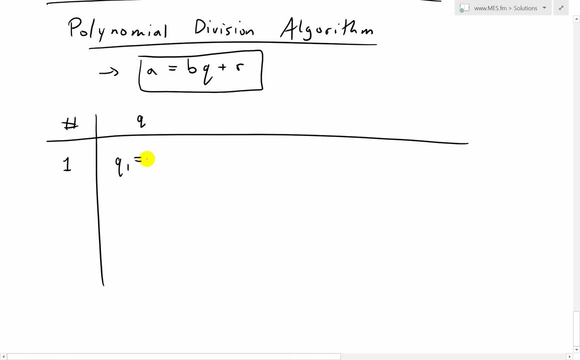 So initially Q is 0, R is A there, So we'll go back. This one needs to always be satisfied, so I'll put that in a box. So Q initially we have Q1 equals to 0. And then the next step would be: well, choose our R So R. you can just rearrange it. 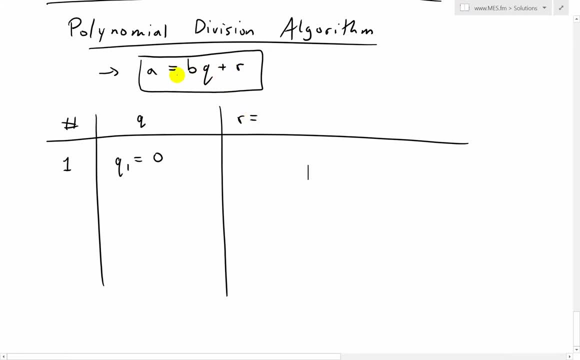 So R needs to, yeah, ensure that this theorem is true always. So A minus BQ like that, yes, we have this part here, And then what we have is, well, R1, plug in Q1 inside, that's a 0. 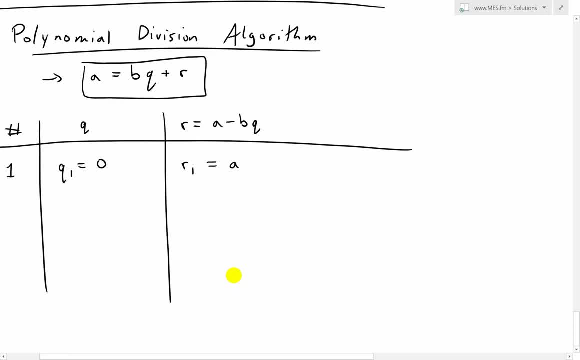 So we have: R1 is equal to A, as the input did in the Wikipedia statement. And then the next column here is: we check if the degree of R is less than the degree of B. right, here Is it, And put a question mark over there. extend this further. 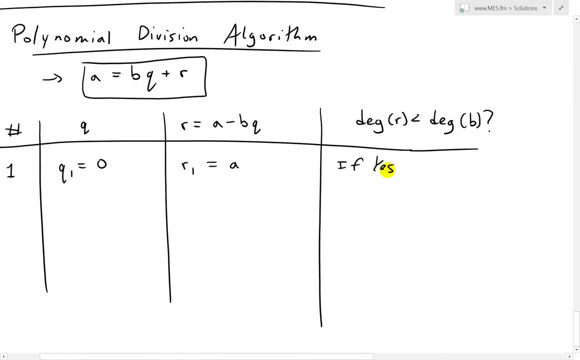 So then I'll write: if yes it is, then we're done. So if yes, we are yeah. if yes equals to done, And we just put that done, Yeah. So if it is less somehow, yeah, then it is just done. 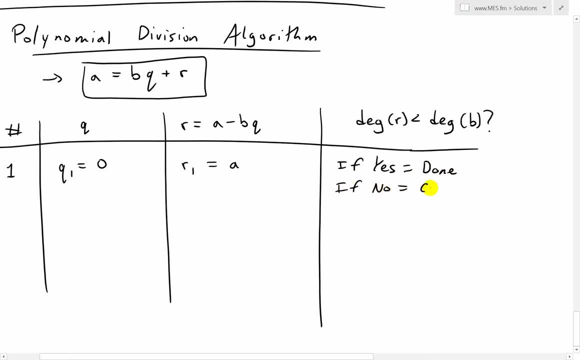 And then if no, we continue. So if it is a no, then that's all good and dandy. So no, yeah. if no, actually before we- what I mean by continue? we add S. this is what the URL right: S1 to Q1. 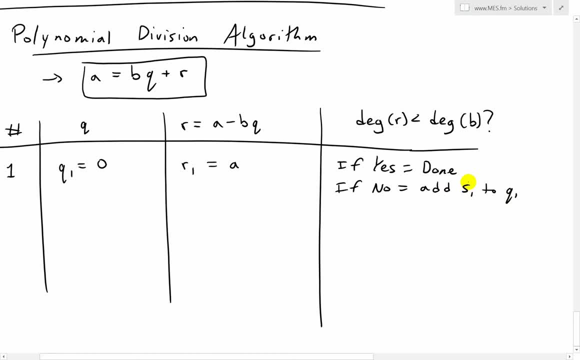 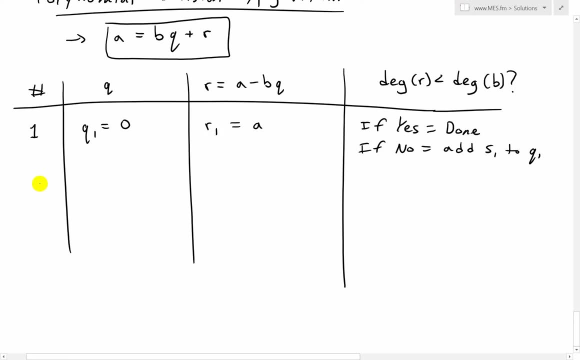 And then I'll explain how the Wikipedia page determines the S1 there, And the reason is we've got to increment it until this one keeps going down and down. So then now we have the second row over here, Row number two. we have Q2 equals to, well, Q1 plus the S1, a new value. 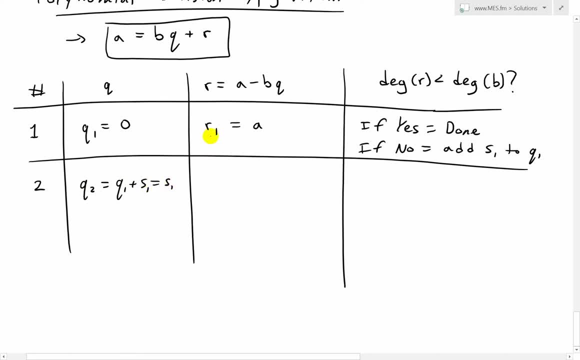 And then that's: Q1 is 0, so that's just equals to S1.. So then this equals here. R2 is going to be equal to. we'll plug this inside, So we have A minus BS1.. A is just this over there. 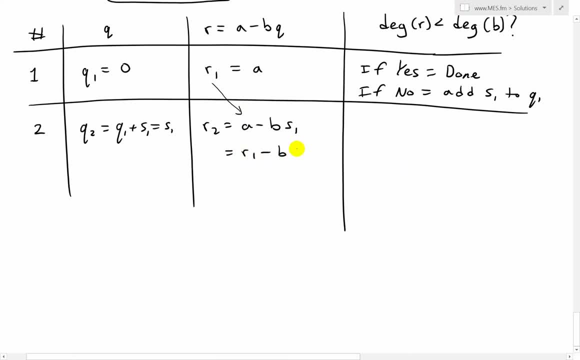 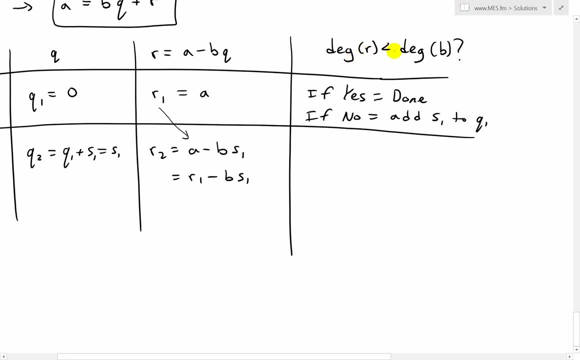 So this just equals to R1.. Minus BS1.. Yeah, so now that we have this subtraction, and now what we have here is, well, we need to make sure the degree of R is less than the degree of B. But we want, so we want to ensure, yes, we want to ensure that the degree of R2, so the 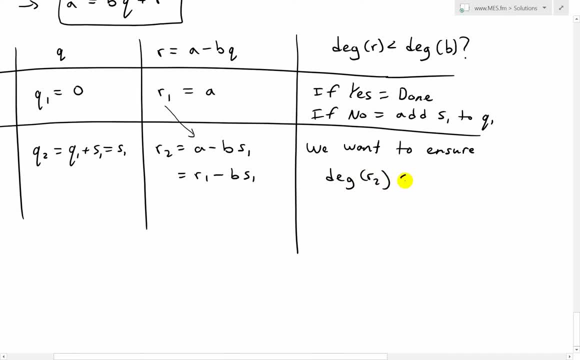 new R degree of the remainder 2, is less than the degree of remainder R1,, so that it's always decreasing. So eventually we'll get to less than degree of B. And then the question is: how do we do this? 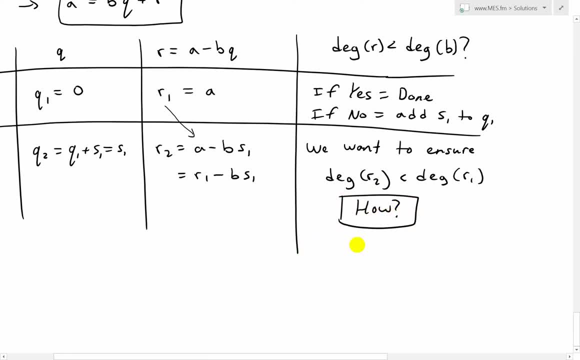 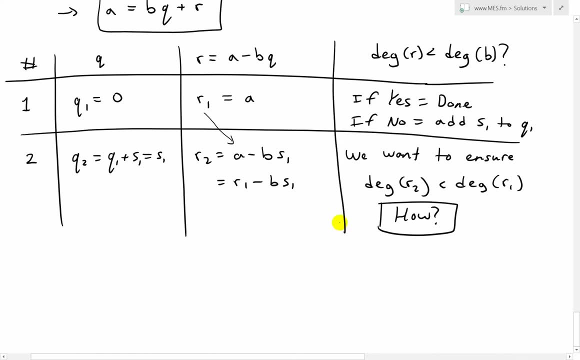 And that is by choosing the value of S1 very specially or specifically to get it. Let's put this a bit better like that. And now what we'll do is I'll just move this down, So cancel this. Let's put this down. 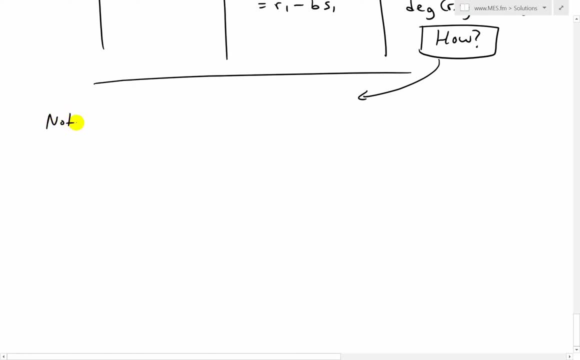 How do we do that? So how do we do that? So what I'll do is I'll write notice First. So what we have, and that thing that we need to worry about, is this: R1 minus B? S1.. So R2 equals to R1 minus B? S1, or, more generally, I'll write more gen early. 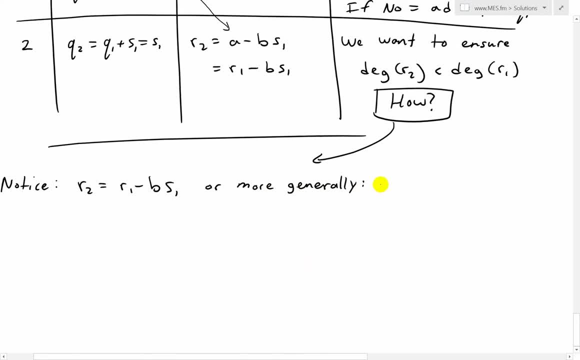 So yeah, basically, or more generally, we'll have it as: instead of 1, I'll put that as I, And then instead of 2, I'll write I plus 1 equals to Ri minus B Si, So the previous one. 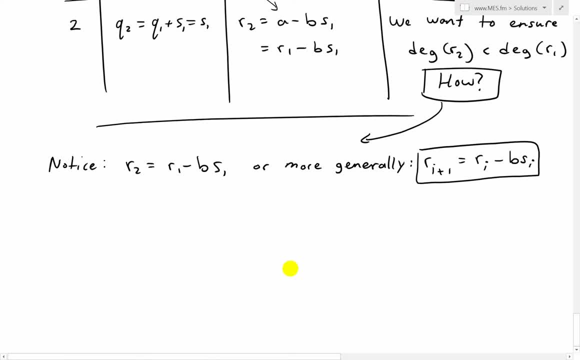 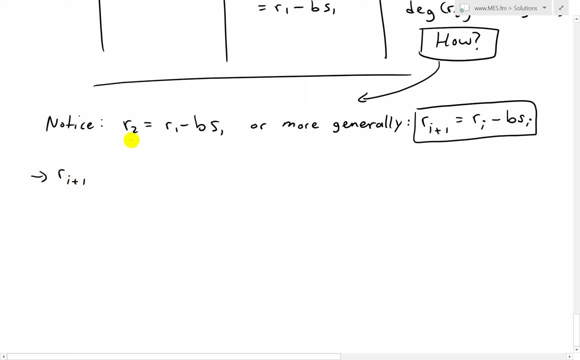 Like that. So, more generally, we have this over there, And now what we could do is write this in the leading coefficient way, So what we'll have is Ri plus 1, instead of yeah, R2, and just write Ri plus 1,. more general, 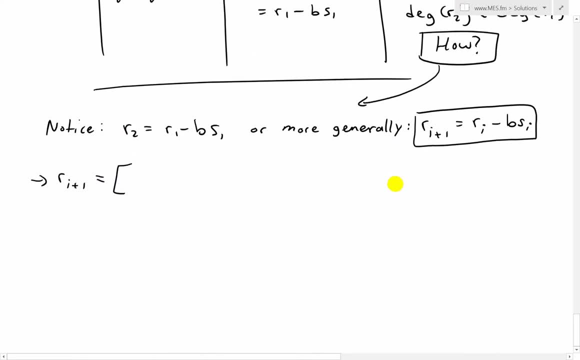 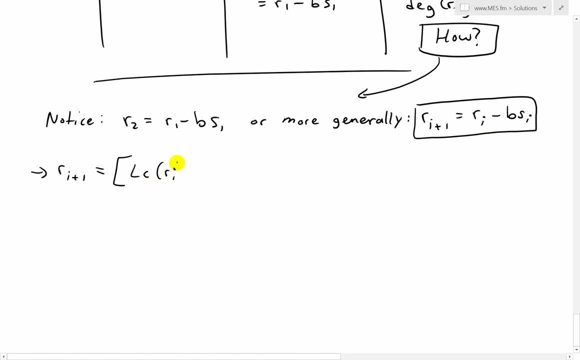 And then what we have is: we want it for every single term to lower, And now what we have is this one here, the Ri. I'm going to write this as leading coefficient of Ri Because, remember, it's just a polynomial Times- it by x to the power of degree. 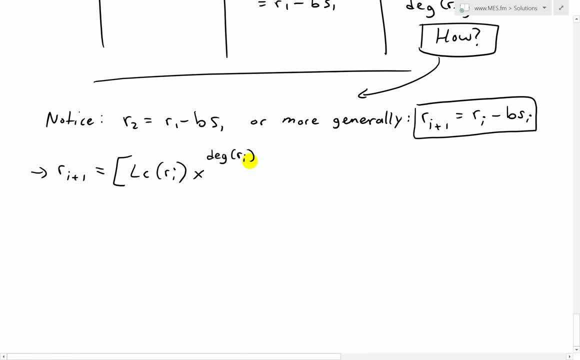 Of Ri, Okay, Of Ri. And then it has plus dot, dot, dot, random stuff like that, the other terms that I don't really care about, because I want to lower the degree of it by 1, so we just put the highest degree. 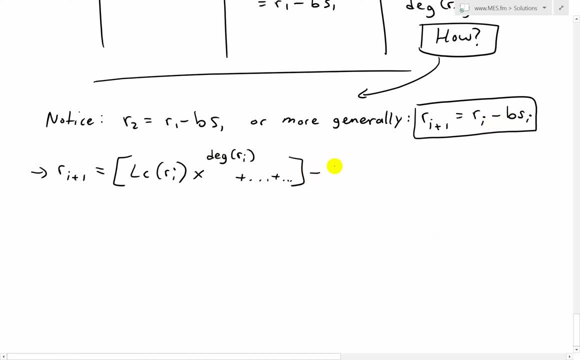 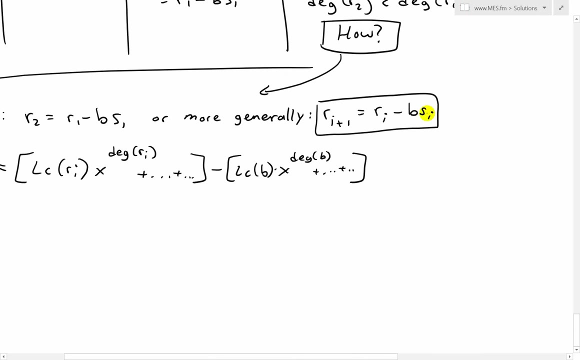 there, And now we subtract it by B, which is going to be leading coefficient of B, times it by x, to the degree of B plus dot, dot, dot, plus, dot dot. and we keep going on and on, And then, lastly, the Si. 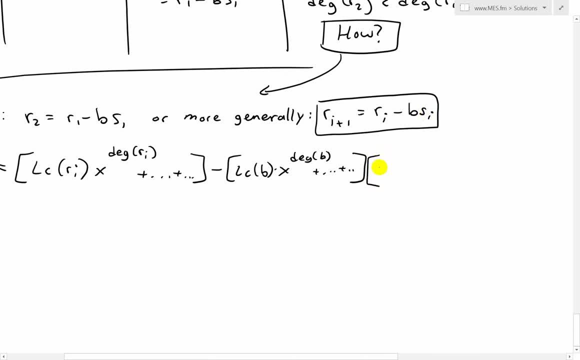 It's still going to be a polynomial. It's going to be adding it to the Q, so we need it to be a polynomial. So multiply the B1 by. this is going to be now Lc of Si, leading coefficient of it times. 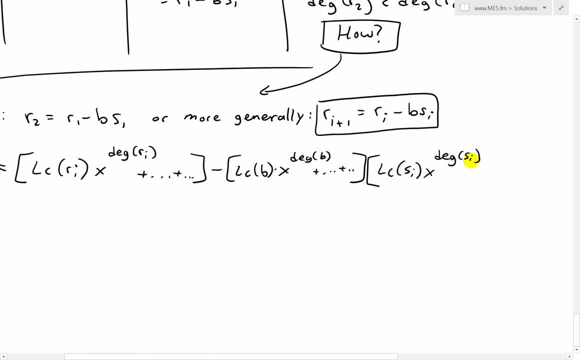 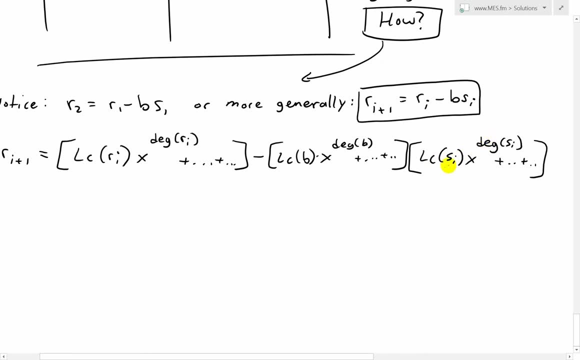 it by x to the degree of Si, Like that, And then plus dot, dot, dot, But I'll show you this eventually becomes: those are just. we get to remove all those terms, because all we need to worry about is lower it by 1.. 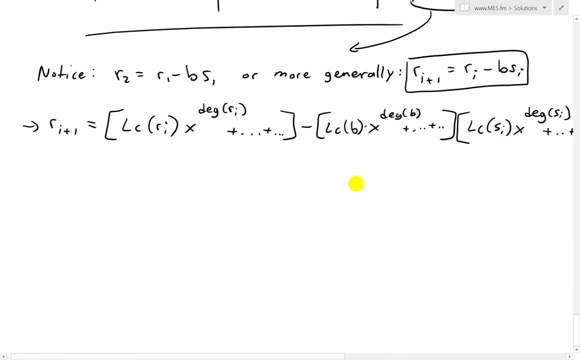 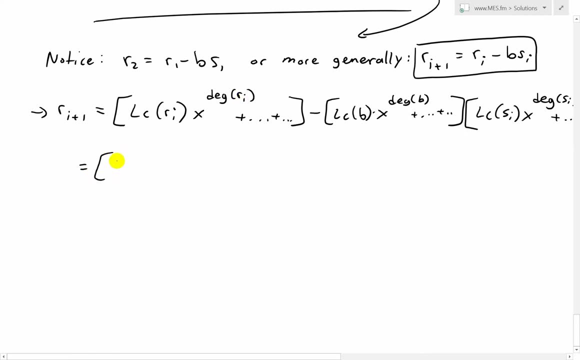 By 1 degree. So all we need to actually care about is this leading coefficient. But this will make sense in a bit, So let's just multiply this out to see what we get. Okay, So this 2, just write this back down again- Lc, Ri, so leading coefficient of Ri, x to 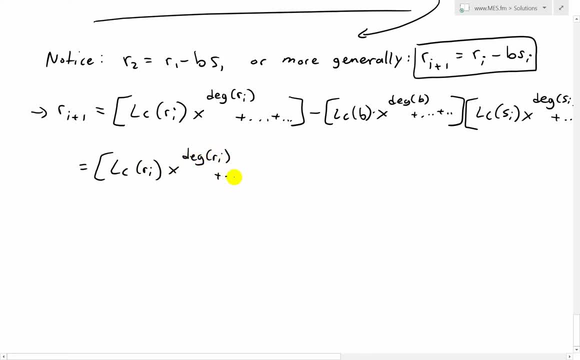 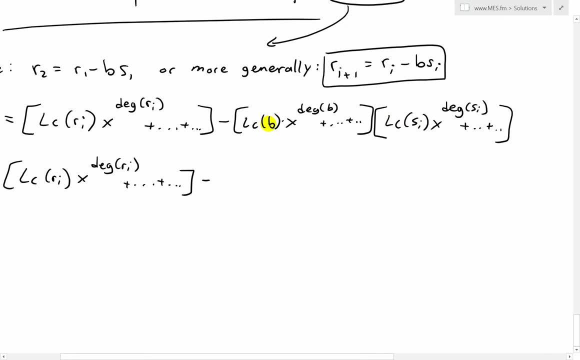 the degree of Ri plus dot, dot, dot keeps going on and on, and then minus. now multiply this inside. So the highest degree that we're going to get is going to be when this multiplies by this. Every other one that you multiply, you're going to be multiplying by, like the B1, or. 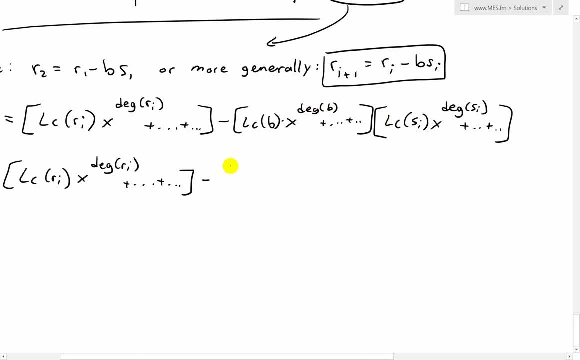 the highest degree by a lower degree, So those don't matter too much. Then what we have is an Lc. It's going to be leading coefficient of B times by leading coefficient of Si times it, by now x and now these just add up. 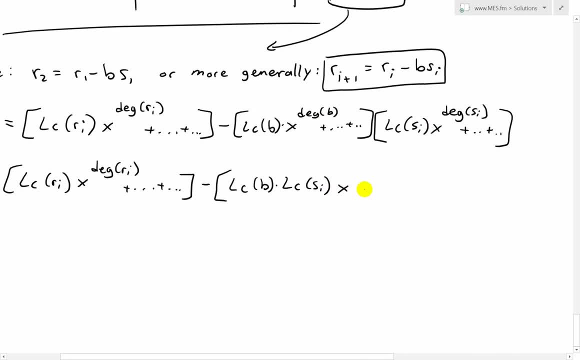 Just like how, when we multiplied the x plus 3, we had x times x is x squared, because those degrees add up. So now we have an x degree of B plus degree of Si, and then we have a bunch of other terms. 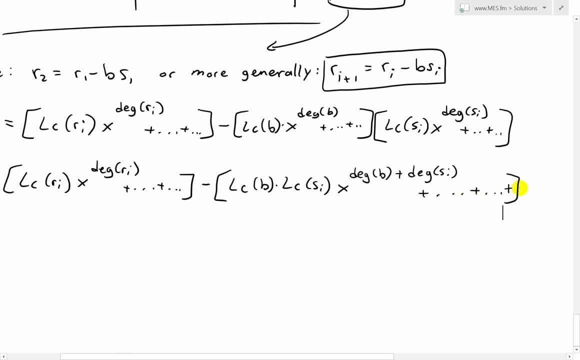 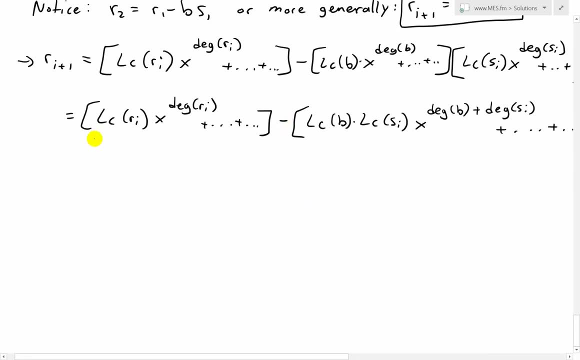 that multiply out, but they all have a less-er degree. Just put it like that. Yeah, so now what we have is: well, we have a subtraction here and we have a highest degree over here of Ri, but what we want is, we want this whole thing and this one over. 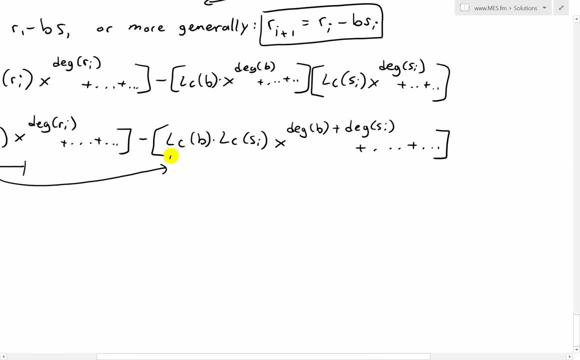 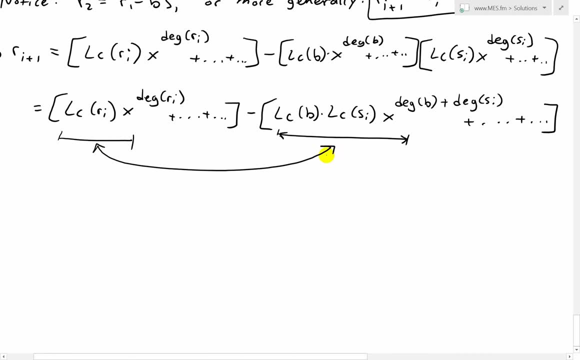 here the highest degree of this term. here. we want these to both cancel, Like that. I'll just put this over there: Want to cancel these? Yeah, So we want to cancel, Yeah, So the reason is yeah. and then this is the reason is so that this degree of Ri vanishes. 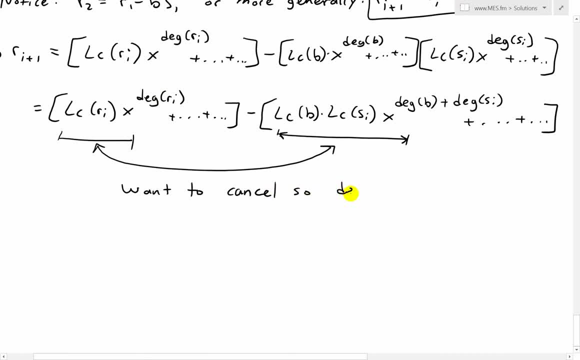 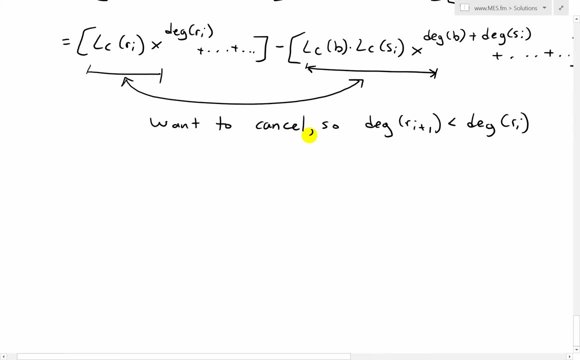 and then we want, so we want to cancel. so that degree of Ri plus 1 is less than the degree of Ri. So we've removed the highest degree there. Yeah, so we want them to cancel, and in order to do that, we'll just make it basically equal. 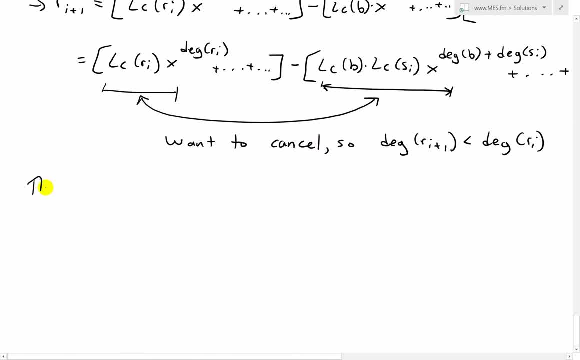 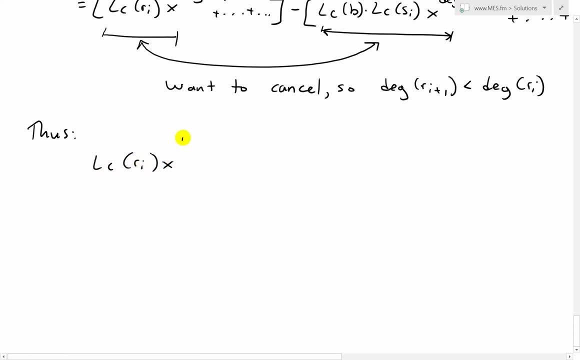 each other. So this is number Ri plus 1.. Thus, the only way it's possible, if they equal each other. that's the only way we're going to cancel LC of Ri. the leading coefficient of it times degree x to the power of degree. 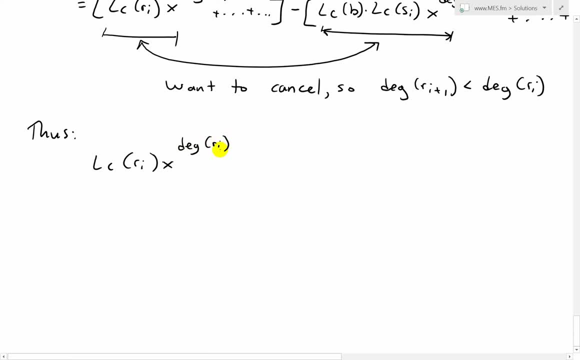 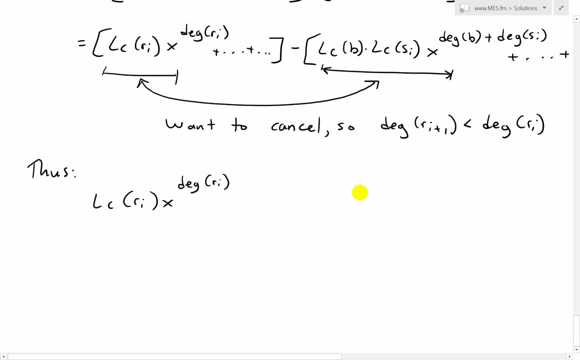 of Ri like this, And then again you have the plus plus. actually, we don't even need the plus plus because we just need to cancel these ones here. These ones just need to be equal to each other. So this has to equal to this. on the other side, LC of B L and then times it by LC. 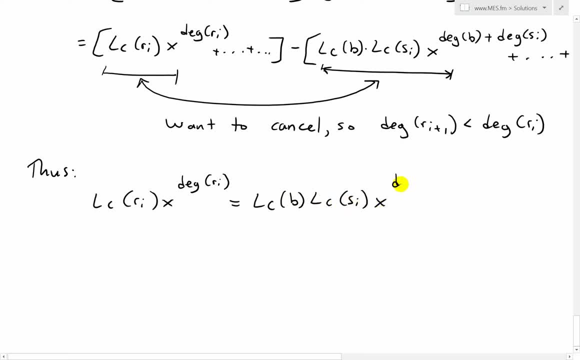 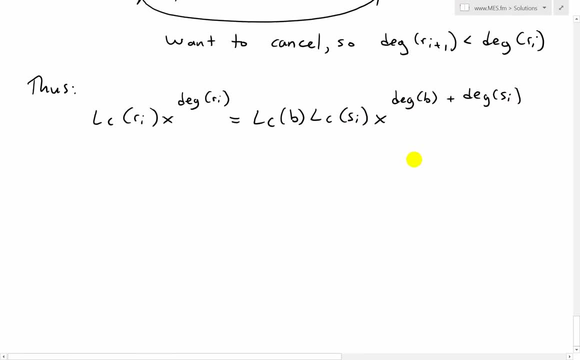 of Si And then times by x, Yeah, x to the degree of B plus the degree of Si, like that. And this is only true if these are equal to each other. So then we have these equal. so we have LC Ri equals to LC of B times LC of Si. 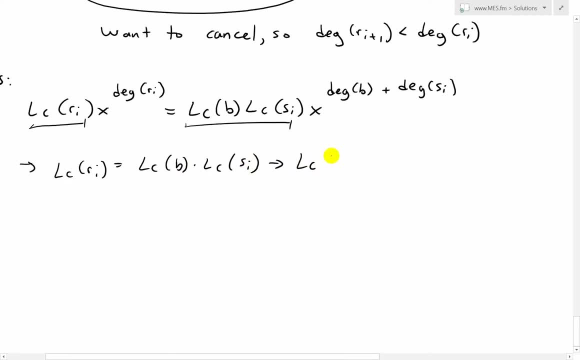 And again, you could just rearrange this, for the LC of Si is the one we want to find out, because we're adding it to the Q. So LC of Si, Leading coefficient of it, is going to be equal to. let's move this over. 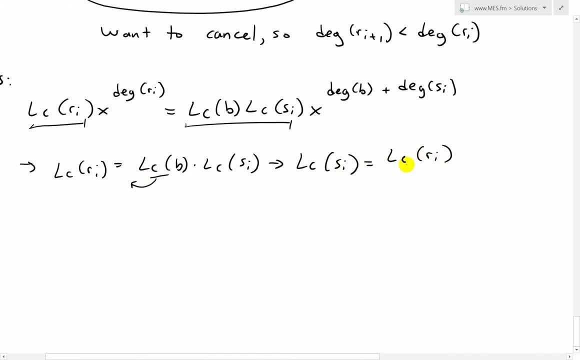 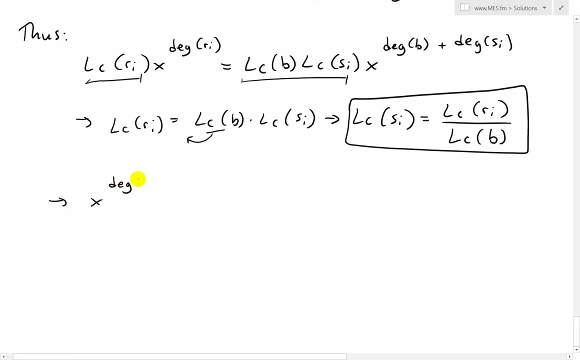 So we get LC Ri divided by LC of B, leading coefficient of it, And this is exactly what is used in the Wikipedia algorithm, And likewise, these degrees need to equal each other. So then, and also what we need is: well, x degree of Ri equals to x degree of B plus. 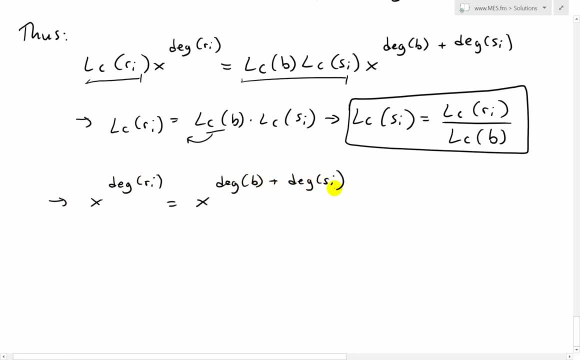 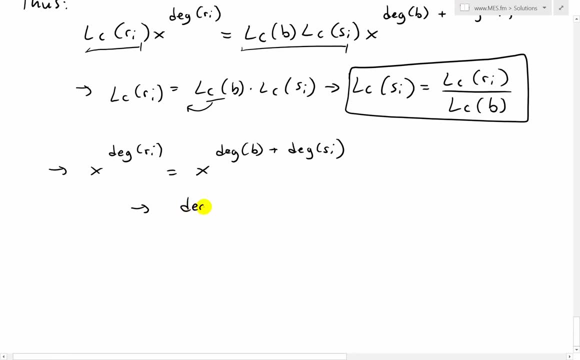 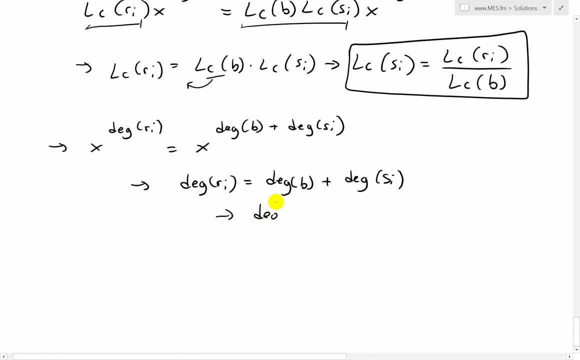 degree of Si: Yeah, Yeah, Like that. So then we have over here these equal each other. Degree: Yeah, So then the degree of Ri equals to the degree of B, plus degree of Si, Like that. And then we could just rearrange this one and we get degree of yeah, so then the degree. 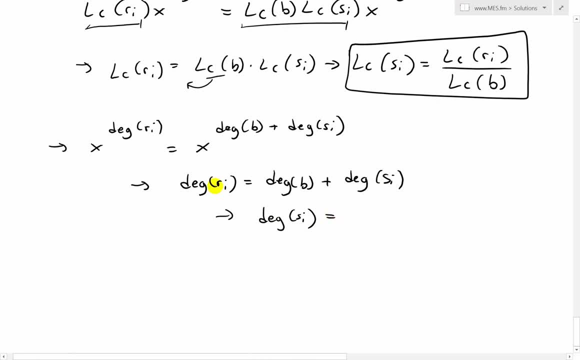 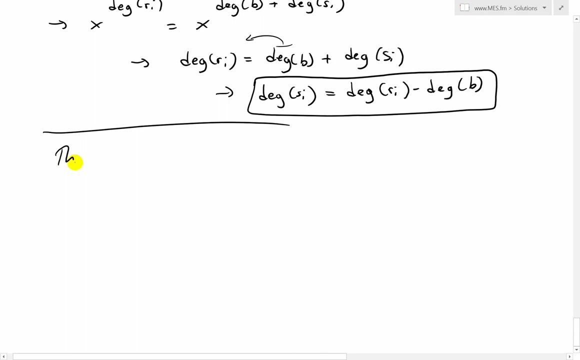 of Si equals 2.. And now what we have over there? No, just move this over to this side and we get degree of RI minus the degree of B. very, very interesting. it's exactly the same thing as the Wikipedia algorithm. yeah, so thus, what we have is all right, thus we choose. so we choose our SI. 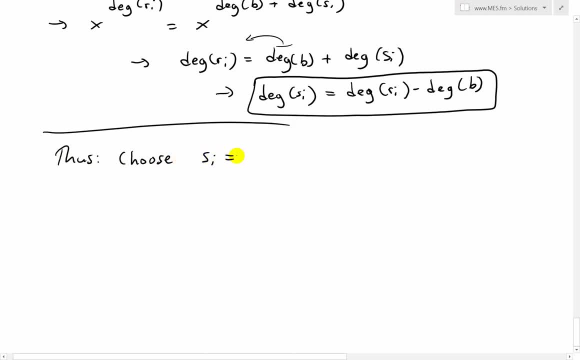 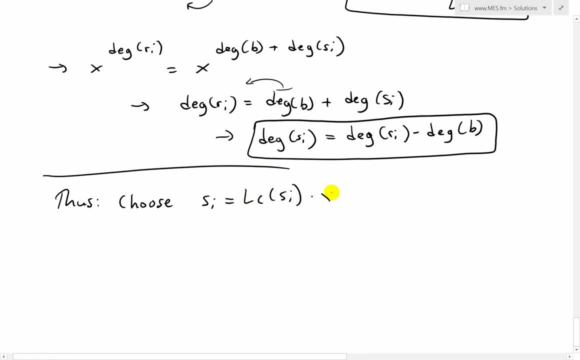 choose, SI equals to this one. here is this going to be? just put the leading coefficient of it, SI, times it by X to the degree of SI, and then we have plus dot, dot dot, plus dot dot. this one. all we need to worry about is, well, it's just to. 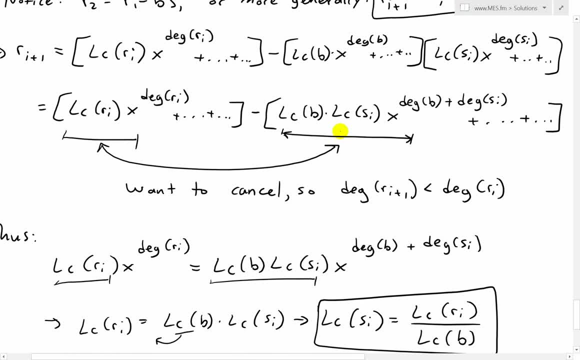 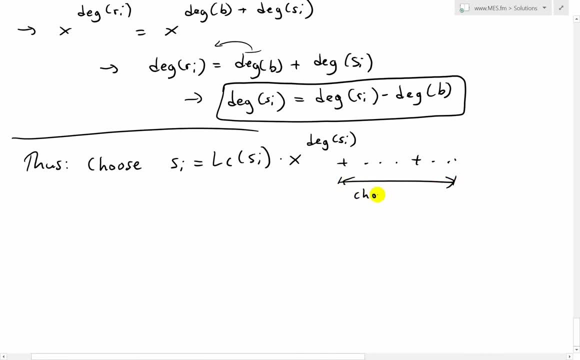 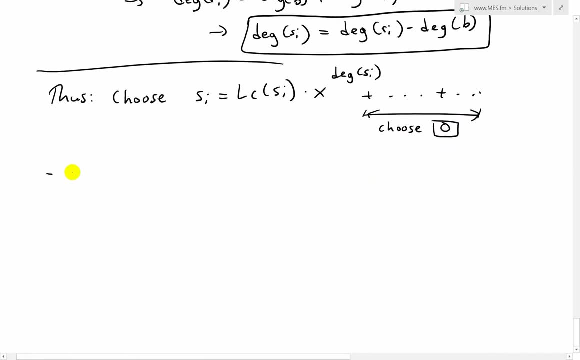 get rid of this leading coefficient or just this whole term. there's all we need to worry about is this. so what we could do is we just need to choose any of them and also write this as: choose this whole term as zero, choose zero. so make it just basically nothing there. so then what we have is SI. 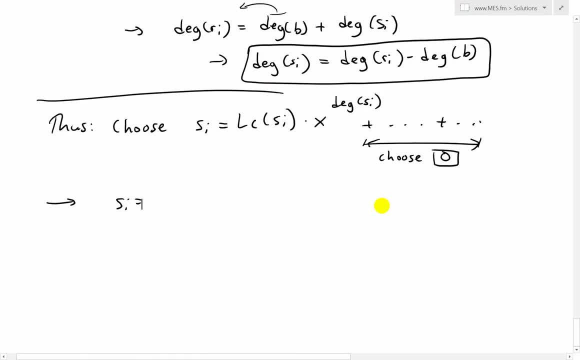 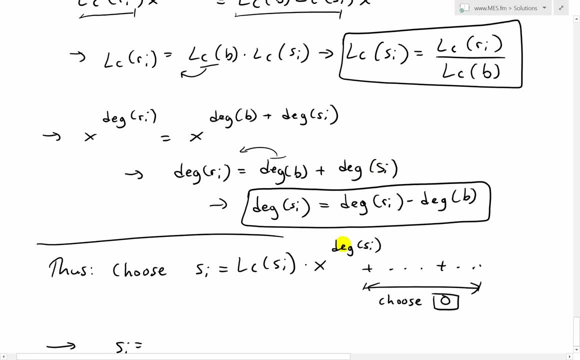 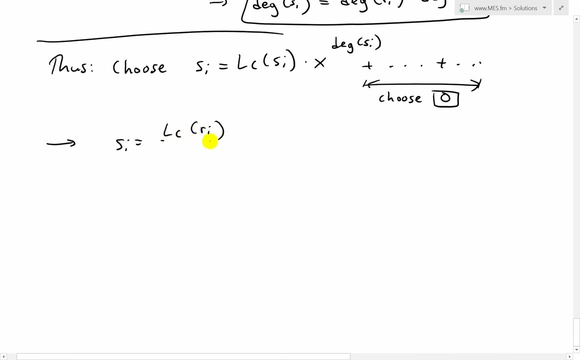 and we replace this by the value that we want is over here. yes, so we want LC of RI equals to. I mean LC of SI equals to this. the difference so we have SI is equal to LC of RI divided by leading coefficient of B, times it by X. 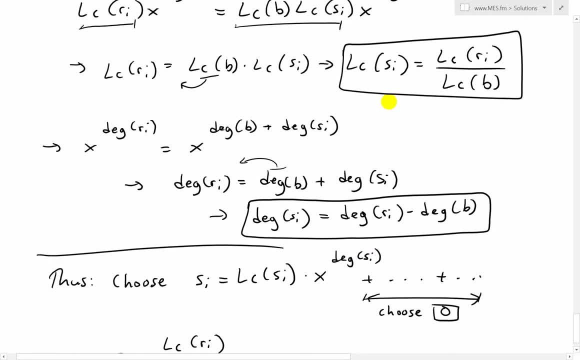 right, so that's what we're going to do, and then we're going to do the same thing over here. so we have X to the degree, and now we have, yeah, this one over here. so we have X. the degree of SI, which is? degree of SI, is just the difference. RI. 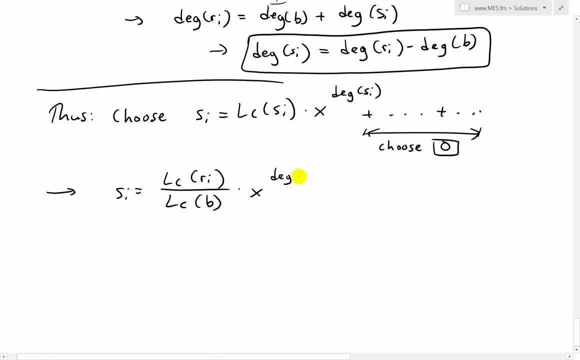 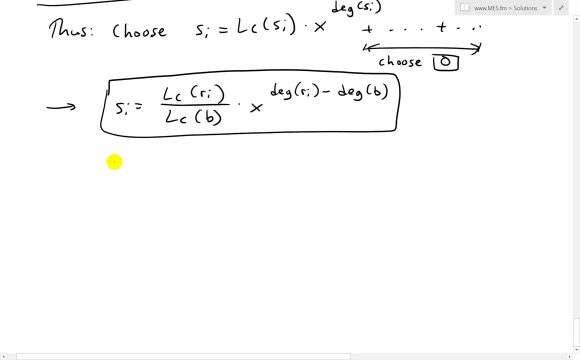 minus B. so X degree of RI minus the degree of B, like this. and then we just choose other part: all equals zero. so then this one right here and this over here, this is what we choose and this ensures, and it ensures that a degree of RI plus one, so the one after is going to be less. 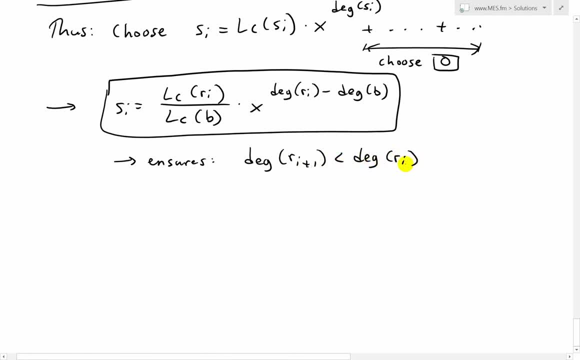 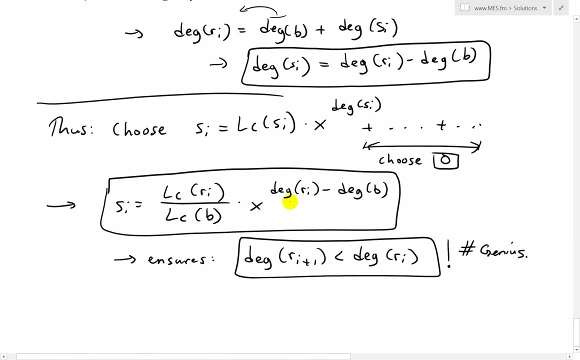 than the degree of RI, like that, and it's absolutely genius actually. this is hashtag genius actually when we work it through. so if we go back up, notice this one, the difference of the RI and B and the leading coefficients, and then the subtraction of that, so the other division there, just to show you it's the exactly. 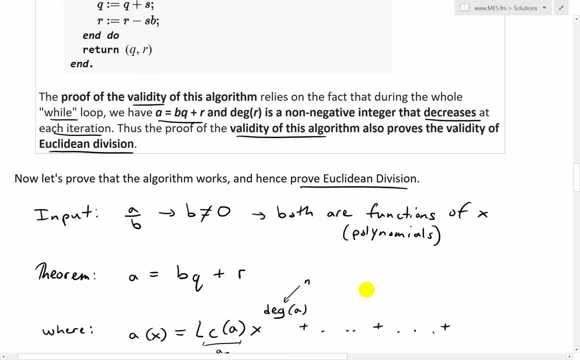 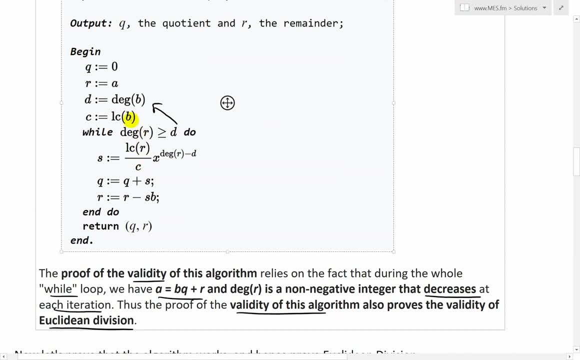 the same one, and that's why they chose S in such a way. so if you go here, they chose: leading coefficient of R divided by leading coefficient of the C is the B one, then degree of R minus and then degree of B there, and it's exactly the. 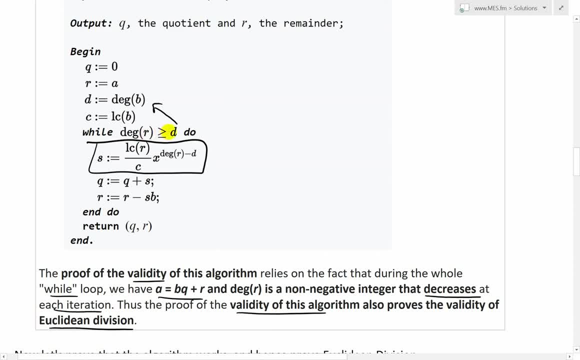 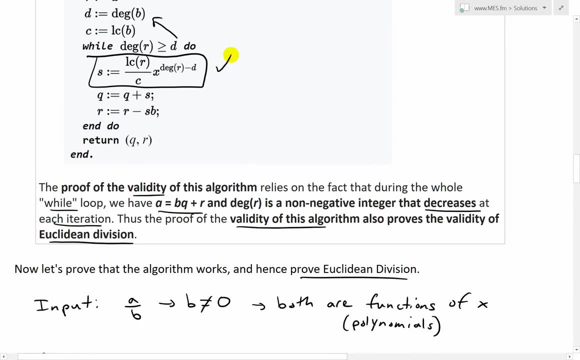 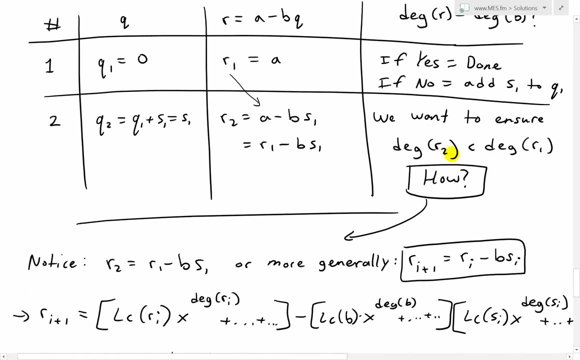 same thing here, and it's the while. this one they have it was if it's greater than it. keep doing this. and so when I just have it, if it's less, stop the same thing and this is exactly the same. one is actually genius algorithm there. and then that is what our SI is, and that's when we have R 2 less than R. 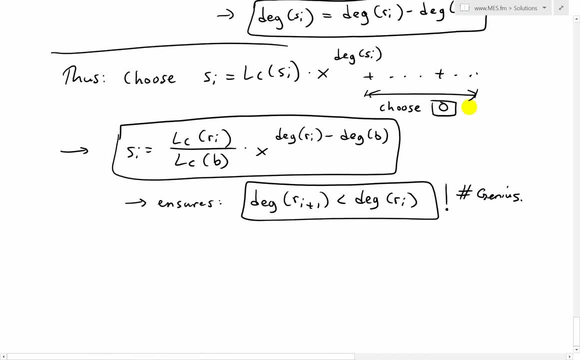 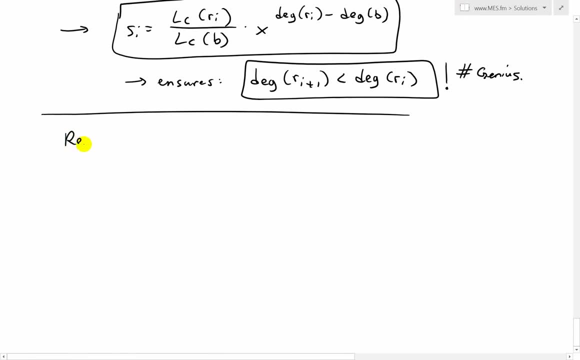 1 and so forth. you keep going on until it's less and less and less. yeah, so now let's revisit the Euclidean polynomial or polynomial algorithm, so revisiting and put that all together, revisiting the Euclidean division algorithm for polynomials like this. let's just revisit it like: 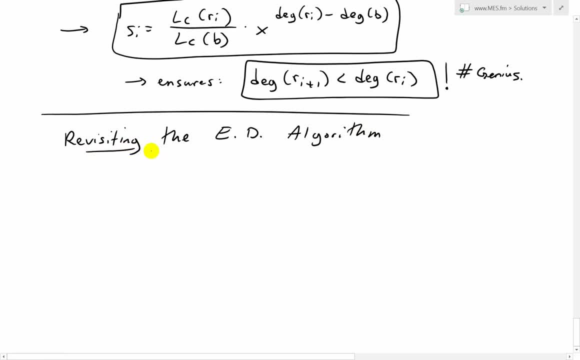 let's put a better underline, underline like this underline and go on. yeah, so, like always, we have our theorem. a equals to B, Q plus R needs to be valid at all times to ensure that we have our theorem works properly, and thus we do. let's just 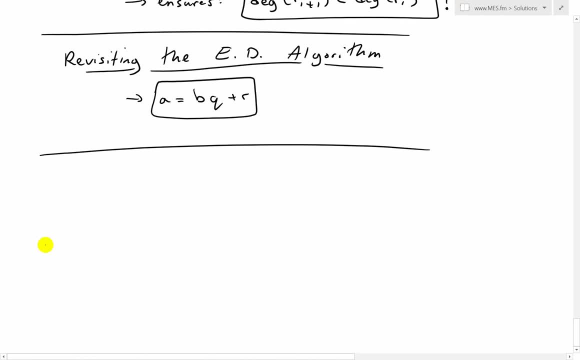 start it again. I'll put this as the question. I mean the, the number of the row. so right row one, we have initially Q like this: now we have here Q, 1 equals to 0, then going further now. so that's initially there. then our R's move. 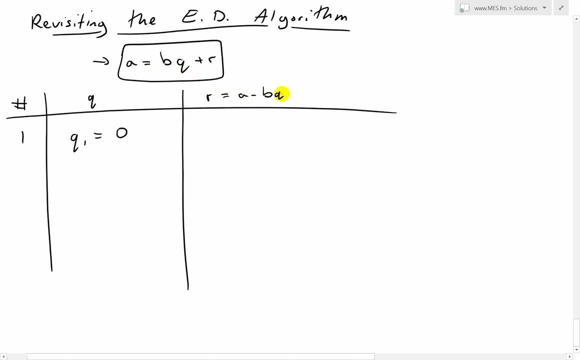 that over R equals to a minus B, Q, like this. and then we plug in our Q: 1 is 0 in there, R is equal to R, 1 equals to a. and now the question remains over here, and then I'll write: degree of R. is it less than the degree of B? like this, so 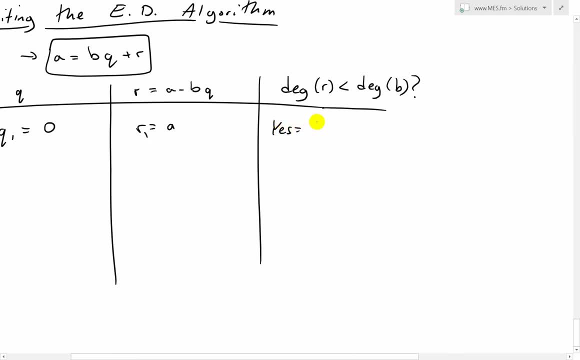 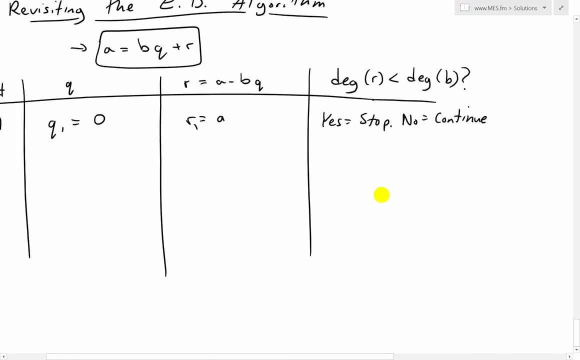 that's the question. if yes equals stop, and then no equals continue, let's put no, yes, yes, equals stop. no equals 2 continue, and we just add the SI to it. so we continue here. number 2 is going to be well, Q 1 plus SI, so Q 2 equals to Q 1. 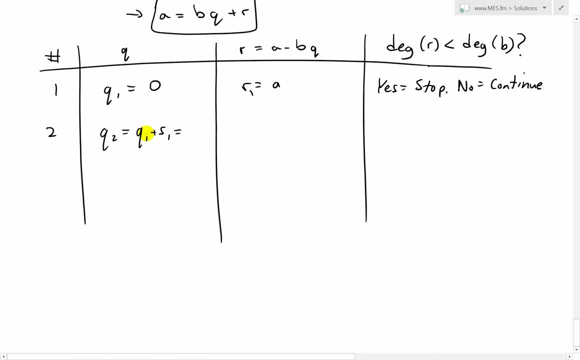 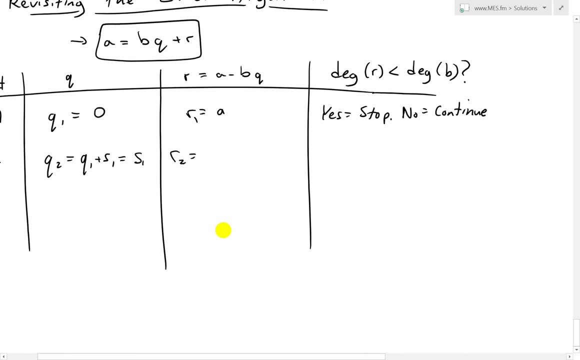 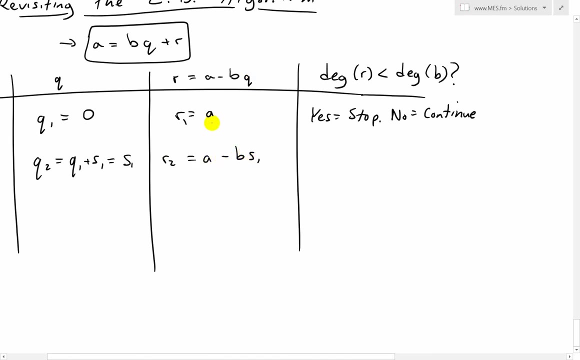 plus s 1, which just equals Q 1: 0, like that. let's just equals to s1, like that. and then r2, remember as above, r2 is just going to be, we'll plug in: s1 in there equals to a minus b s1. and then this a is just over there- equals to r1 minus b s1. and 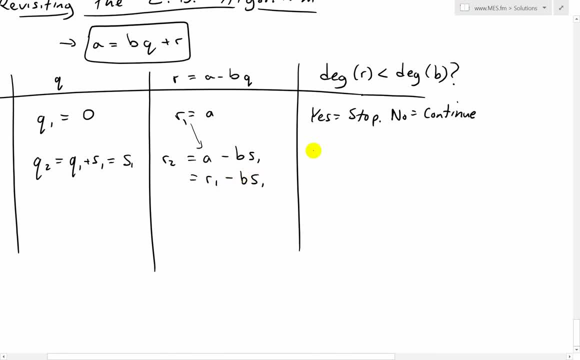 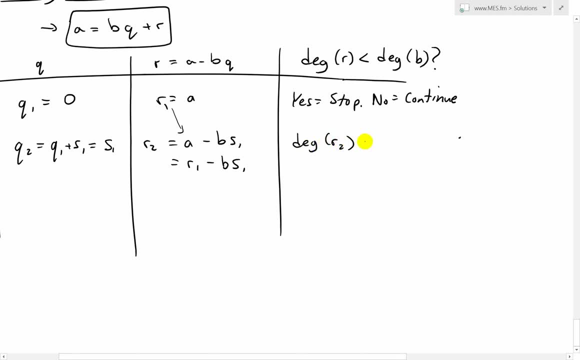 then these subtract, and then we remove the highest power, and here another, we have this one, and then here, as i showed before, the degree of r2 is well less than the degree of r1, and then so on. now we just check if it's less than b. if it's yes, we stop, if it's no, we continue. so dot, dot, dot, and this one. 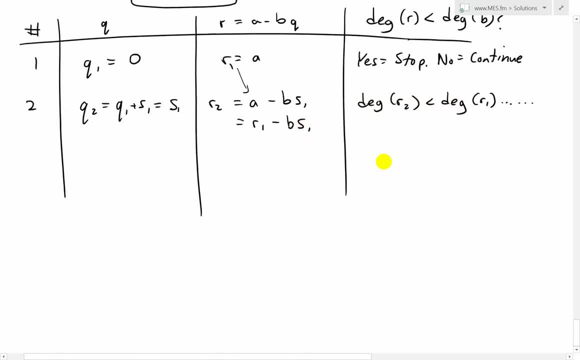 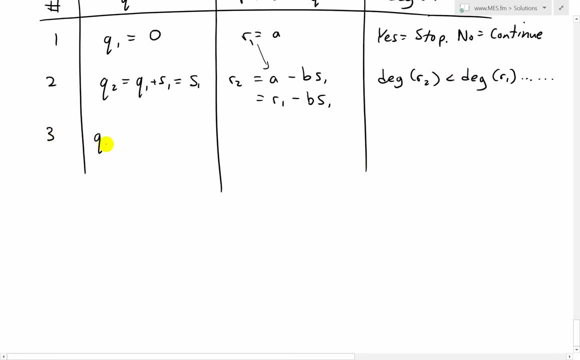 here that that s1. the way we chose it. we always ensure that the next r value or next remainder, always less degree than the other one and eventually be less than b. then now next step: here we have q3, equals to well, we just add, add another s value, so s1 there plus s2, so it's the second one based on the previous value there. 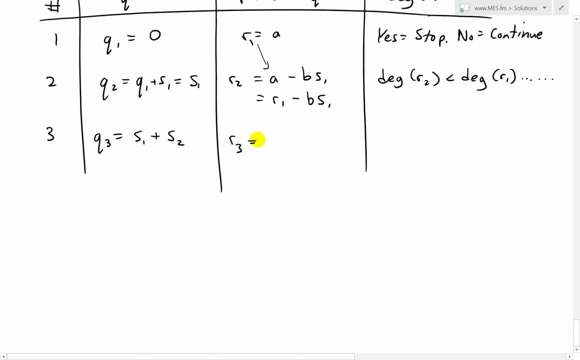 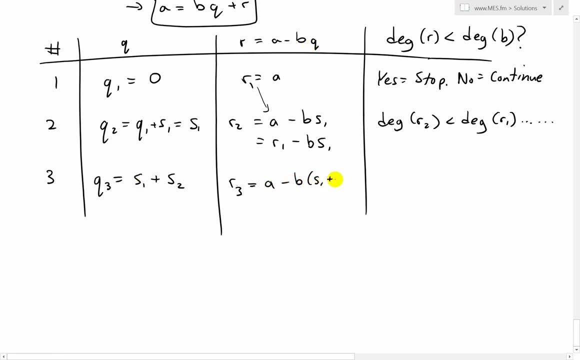 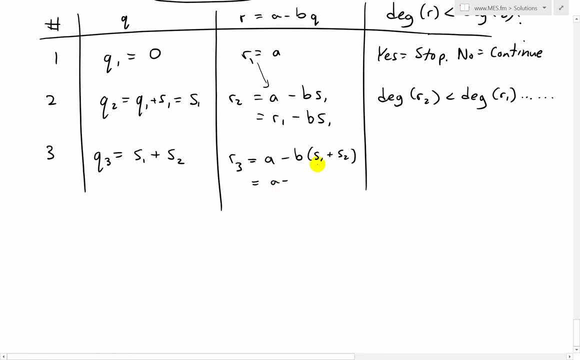 so then we have r3. now this equals to: we can just plug that in a minus b times q, which is s1 plus s2. just show you what we get. a is our, our value there. so this one just going to be a minus b, s1 plus or minus. 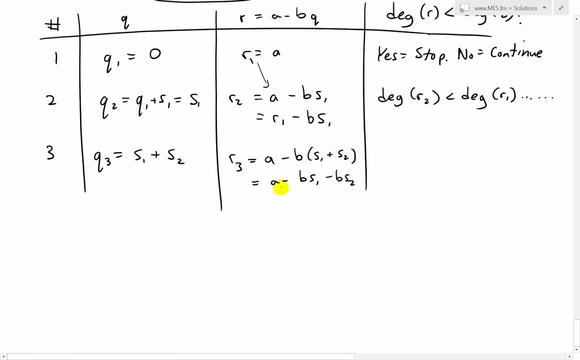 bs2, so this bs1, this is just our r2. this just equals to r2 minus bs2, so we always subtract. so then the r3, like here, it's always going to be the previous r minus the b times s and then the s2. 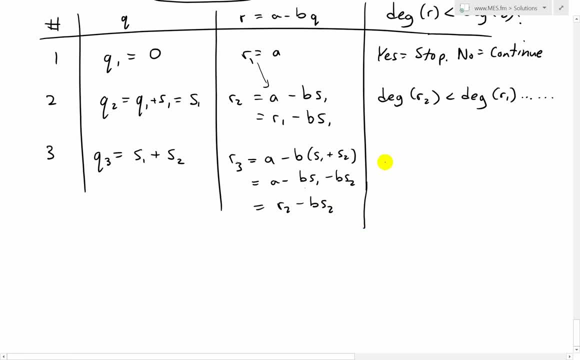 like that, or the previous one like that, and then here as well, we have: degree of r3 is less than degree of r 2, and so on. now we just keep this method all the way until we get to k. so here, the kth row we have: 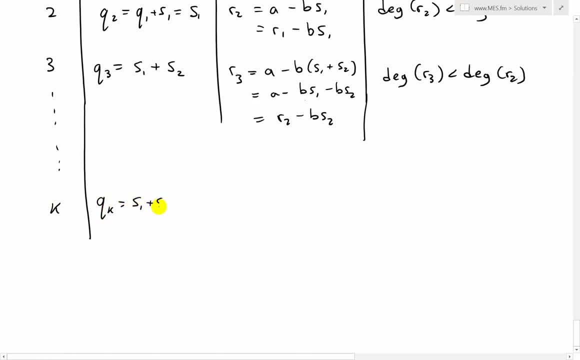 now q of k is going to be equal to s1 plus s2- it's always one less. so plus dot, dot, dot, and then we get eventually s k minus 1. so the previous one there and likewise here. this goes all the way down down here until we get r of k, which is going to equal to r k minus 1, and then minus b s. 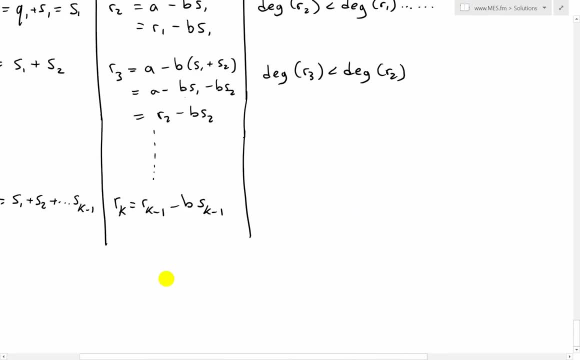 k minus 1, like that over there. and then this is the kth. one is eventually, eventually here, because if we're always decreasing, uh yeah, eventually degree of r k is less than the degree of b, and then and basically we've proven the algorithm, yeah, and basically we have all the way down here. 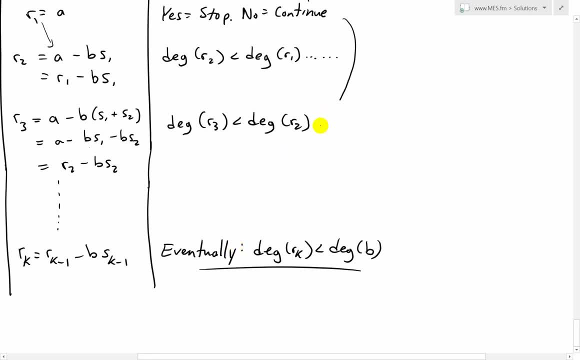 these are all. i'll put this all like this, decreasing. i'll put it actually over over here: put dot, dot, dot and uh, just put an arrow, like this: decreasing, decreasing degree of r, like this, or r i? so it keeps getting less and less and eventually just 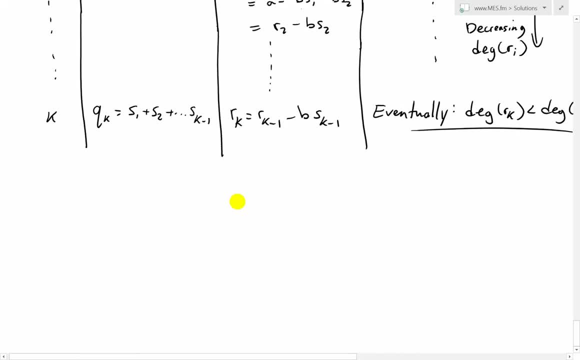 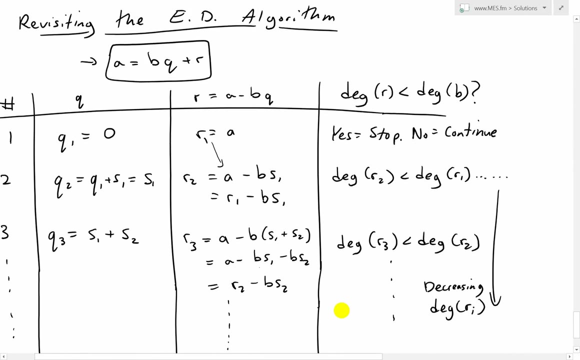 less than the b over there. so then, thus, this proves, and i'll write thus: uh, this algorithm is valid, i'll gore is um is valid and since it's valid, the theorem above has been held. uh, it's been basically taken into account the entire time, and the degree is always getting less and less. 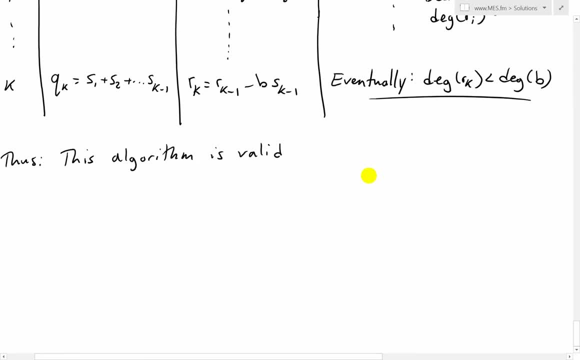 which will eventually get less than b. so less is algorithm is valid and thus thus the把 euclidian uh division. so the e, u for polynomials or the, the theorem is dont e, u, o intended is called is economic rt. so then this should be the amount of things that's needed to be putol: W, lq 1, r showing them. but that doesn't really understand that as of date is it? percent should be the等 n. nobody really gets less than the b. so therefore this algorithm is valid and thus thus the euclidean uh division. so the E, u for polynomials are the, the fermatical. 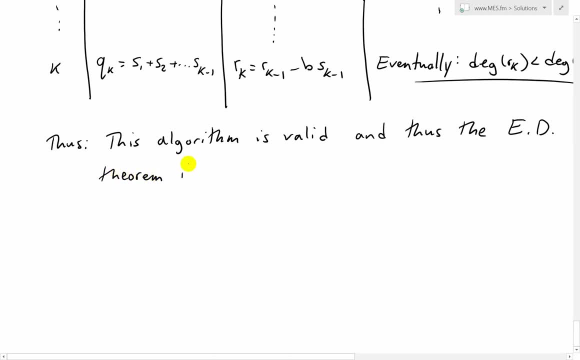 is equal the 49 and the Mash meters here, or something little above the e, 6, u for polynomials are the. the theorem is correct. division theorem is proved so because we proved this algorithm. thus it's proved. hashtag amazing is actually quite an interesting proof where we 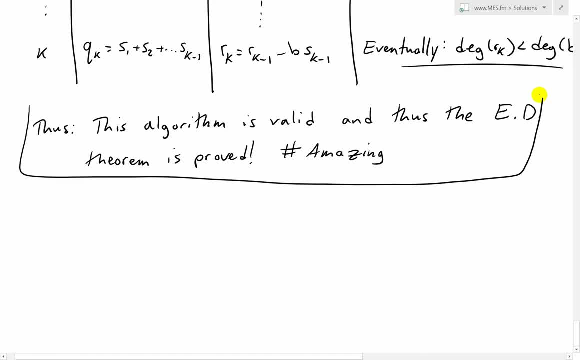 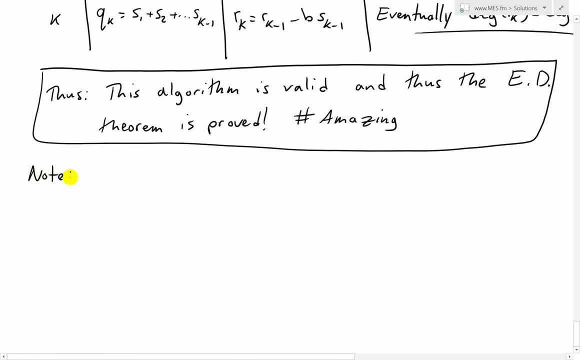 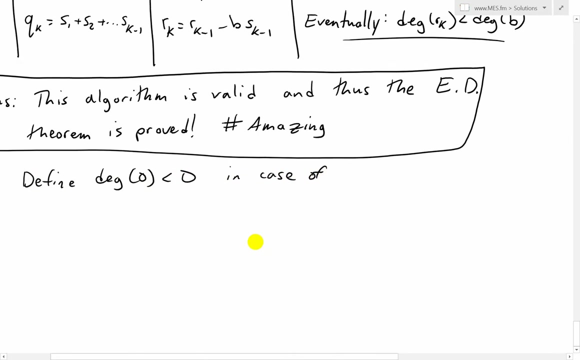 prove it by proving the algorithm instead of just a conventional proof type method like that and over there. and then again, note as the Wikipedia does note: it defines all over here: define degree of 0 as less than 0, and this is in case, in case of, or in case when the degree of B is equal to 0, in case when 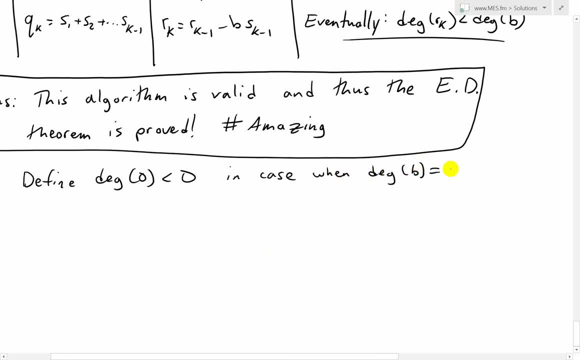 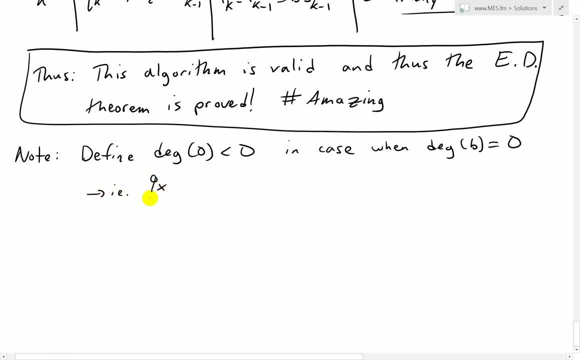 degree of B is equal to 0, and an example of this is: ie. if we had something like: let's say we had 9, 9 x polynomial divided by another polynomial, three is still a polynomial. this equals to our a over b, and then if you just divide it out, that just equals to 3x over there. now if you multiply both, 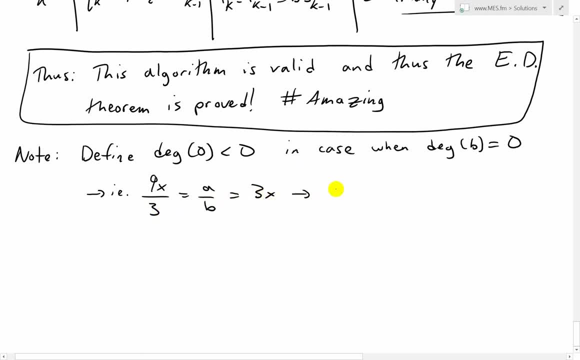 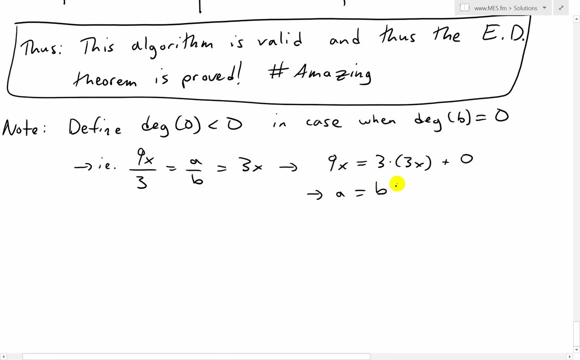 sides by uh three on there. what we end up getting is 9x. well, this equals to uh three. times it by 3x, and then we'll have a remainder play a plus zero. that's going to be so. then we have a equals to b as a divisor. times it by q as a quotient plus r here. so then what we have is r is equal to zero. 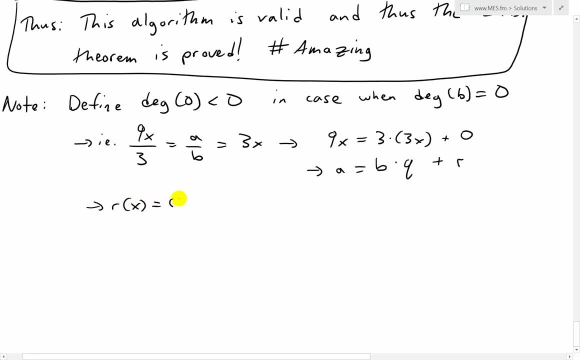 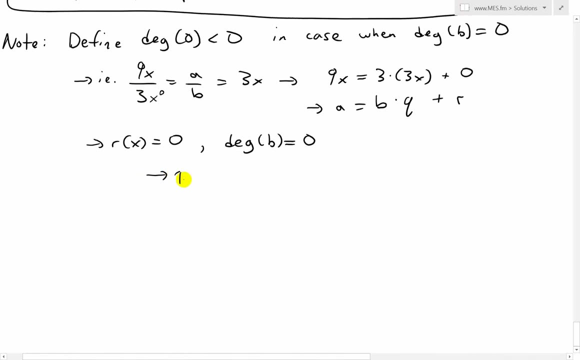 so we have r of x equals to zero and the degree of b is equal to zero, right here, because that's just degree of uh, yeah, x, zero, yeah, that's just three. this is a constant. so then we have to define for the algorithm purposes to keep it going, thus: uh, yeah, thus define. 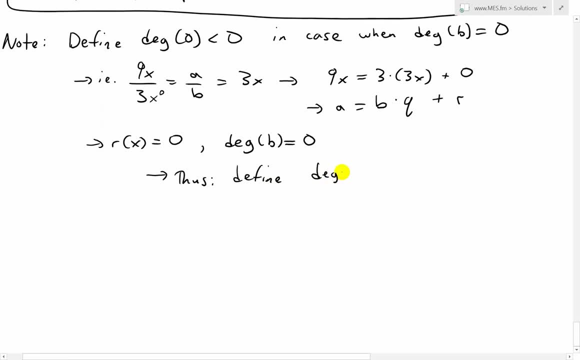 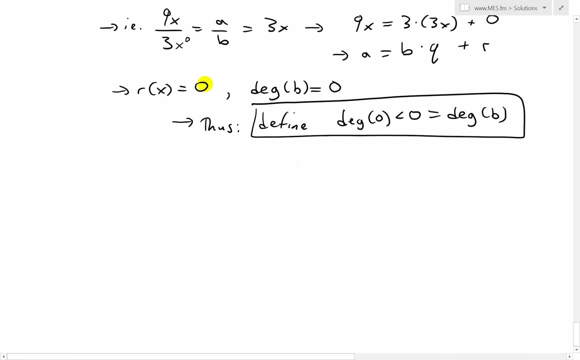 uh, degree of zero is less than zero, which equals to the degree of b in this case. so that's why we have that case there, just make it less, even though technically they're the same degree, because they're both constant: zero, still constant. so now, just to illustrate all this, let's go revisit that. 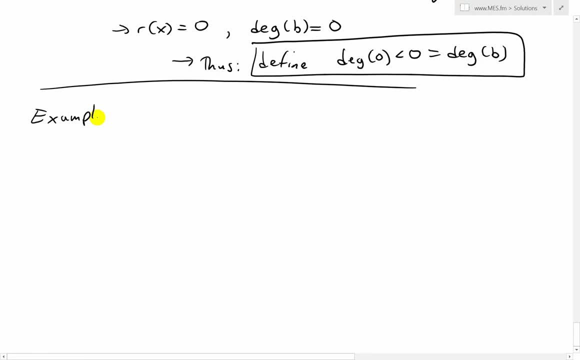 same example of that uh, one above. so let's use that same long division one uh. but now we're dealing with the uh, this individual chi um, including division. so x plus three squared, now we have the two x plus two. this equals to again expand that x squared plus uh, this three times, x plus x times. 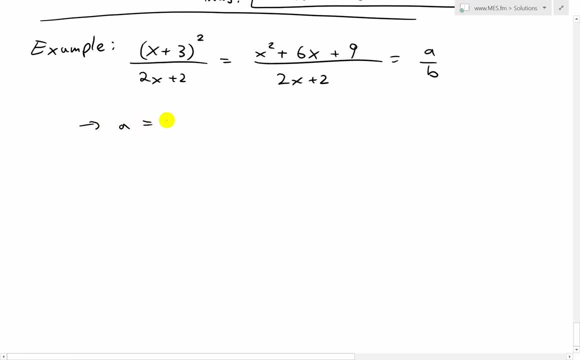 we always need to have a equals to b, q plus r. so that's the clinton division. now what we'll do is make the giant table like this: put row number here and i'll write row number one, and then we have our q value here. q1 equals to zero. and then next one we're going to do is: well, we need to 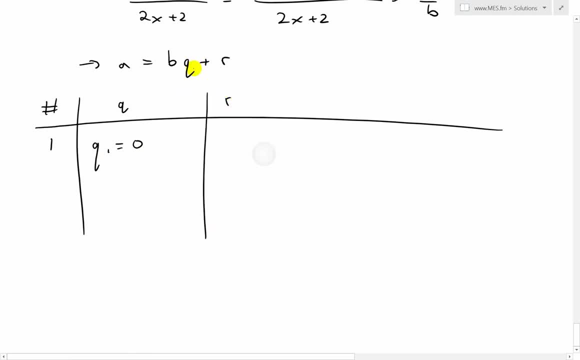 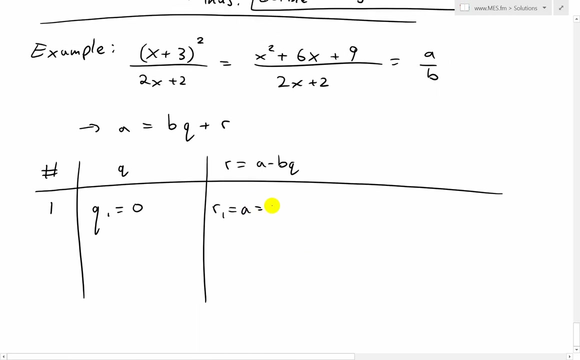 determine our r value. so r- just move this over- equals to a minus b, q. so r initially is going to be r1 equals to a right here. or i'll write this out like this: r1 equals to a and a is just the top one there. equals x squared plus 6x plus 9, like that, and now the degree. now we do the check. 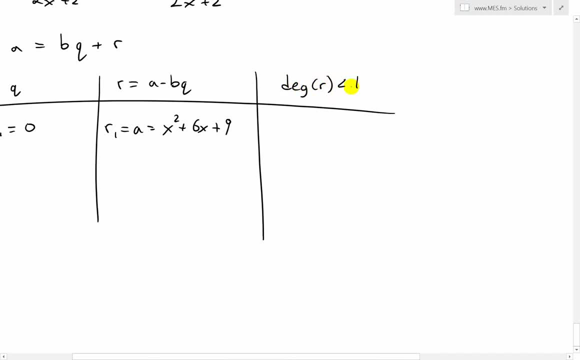 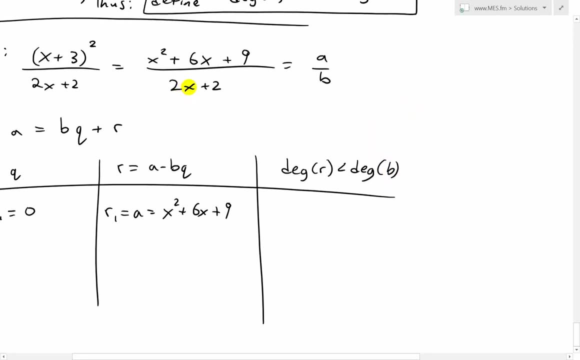 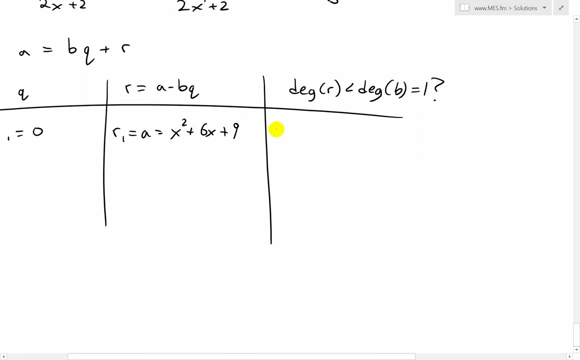 is the degree of r less than the, the degree of B, like this, and in this case, here the degree of B is 1. this is 1, which equals to 1, is it? and there's the question. so then we check here: degree of well, or here, degree of r1 equals to 2, which is greater than 1. so we do know. 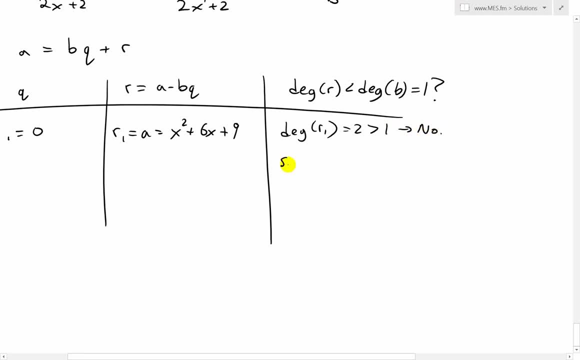 right here. so now we have to choose our s1 value. s1 is going to equal to number leading coefficient of r1. so LC of r1 divided by LC of B, times it by x, and then the degree of r1 minus the degree of B, like that. and then now, if we write: 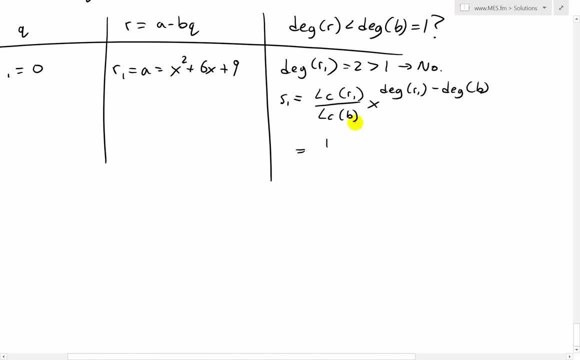 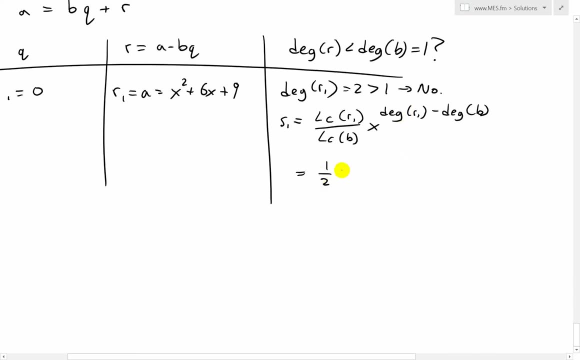 those out, LC, this is going to be well 1 there. so if 1, then degree- I mean leading coefficient of B- is 2, that is LC of B, that's 2 and then X, then the degree is equal to D and super 1. and then if we divide up this equation and these. digo Bizhull, käyt có text. and this equation becomes 0, that's Q, that's equals to dealers, cube times the catch number 2, station square Fuller's exponents. then we say here: D Euro, this is equal to 16, that which equals to 16, and then we do: 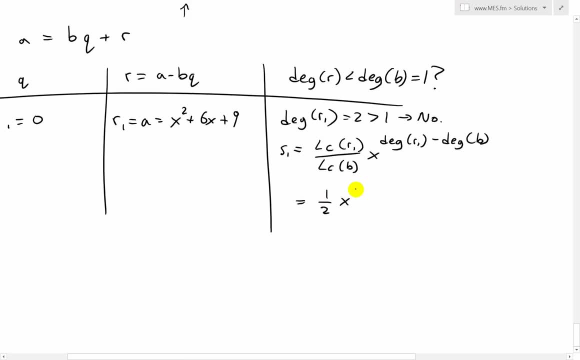 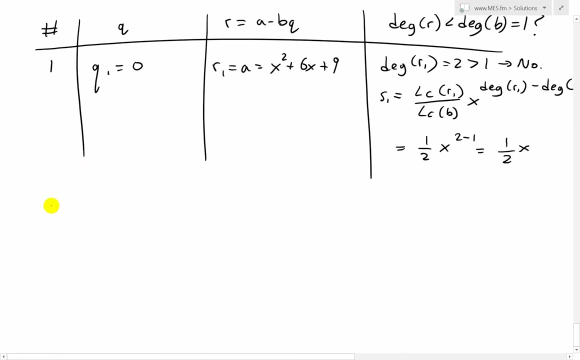 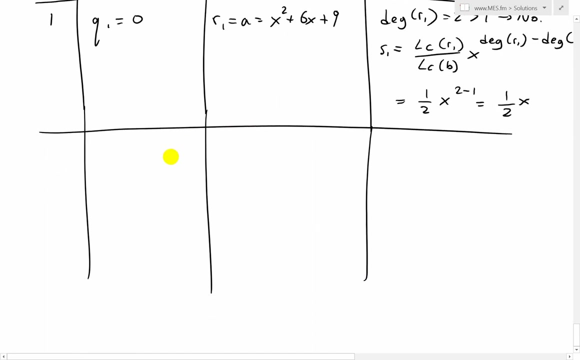 Degree of R1 is 2, so we have 2, minus degree of B is just 1, like that, this just equals to 1 half of X, so that's our S1, so then now we have that part set up, and I'll just write this out like this and then expand this out, and now we have Q, that's Q1,. I mean now the second row. I'll write this as number 2, over here. 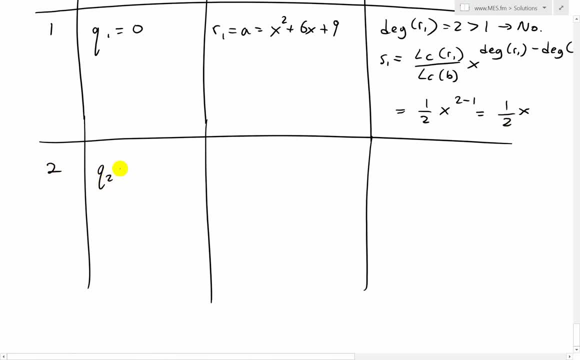 and then the Q2, we add S1 to it. this equals to just S1, and this equals to: over here, this is going to be plus, yeah, that's S1,, which equals to 1 half X, like that. or I'll write the Q1 plus S1, just for completeness, and this is 0, this is just going to be 1 half of X, like that, and then we subtract it. so now we have R2,. 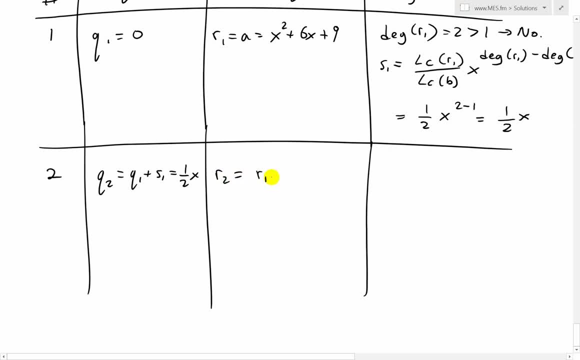 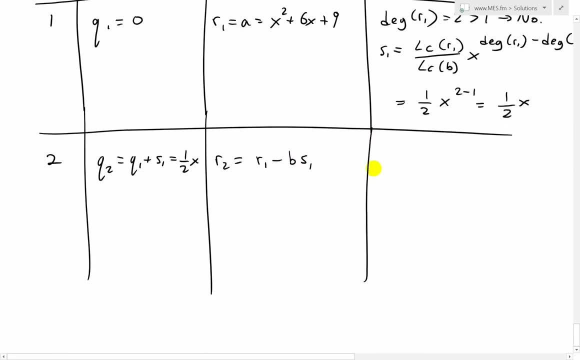 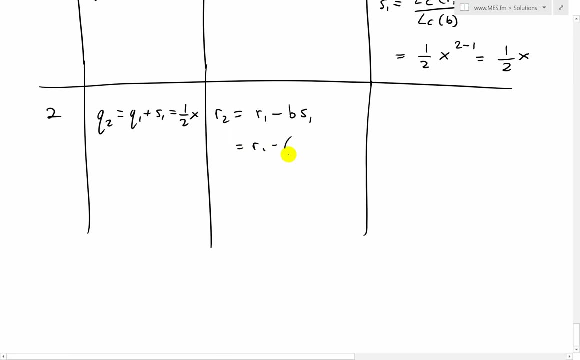 so R2 is going to be equal to R1 minus. now we have B, S1, like that again, you can plug in those values there and you'll get the same thing, and then the S1, so R1, I'll put this all actually, before I do that, I'm just going to expand this out. so B is just 2X plus 2, and then S1 is 1 half of X. so when you multiply that inside, what we end up getting is well, we equals to R1,. 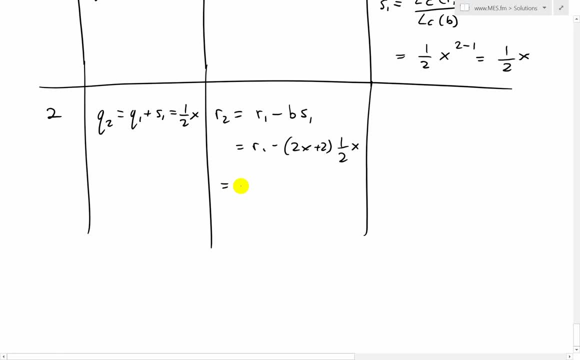 so let's write the R1 first, so this equals to R1, is the X squared, that's just above here, plus 6X plus 9, and then now we have here: minus 2X times 1, half X, the 2's cancel. we just have minus X squared. and then here again, minus 2 times X over 2, the 2's cancel, minus X, like that. notice what we have here. this cancels with this. 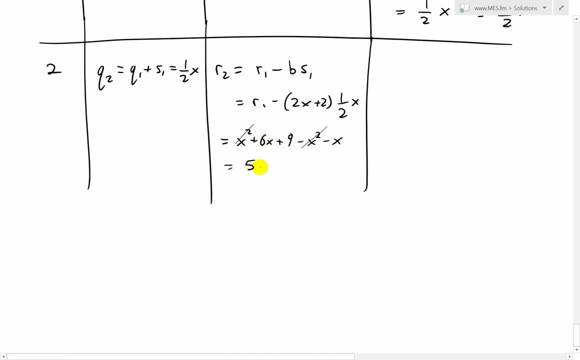 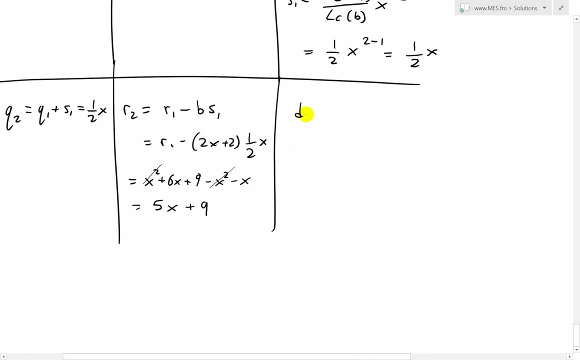 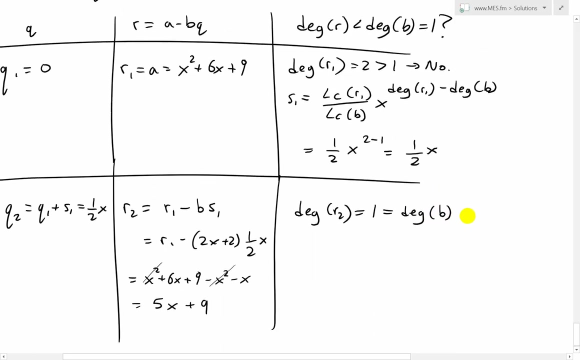 and then this one in here, and then we add those up. this equals to 5X plus 9,, like that. exactly as long division where we had 5X, 6X minus X is 5X and we carry the 9 down, we have 5X plus 9, and now we check again. this is degree of R2. equals to 1, equals to 1, which equals to degree of this is going to be B, like that, so it's not less than it equals to it. 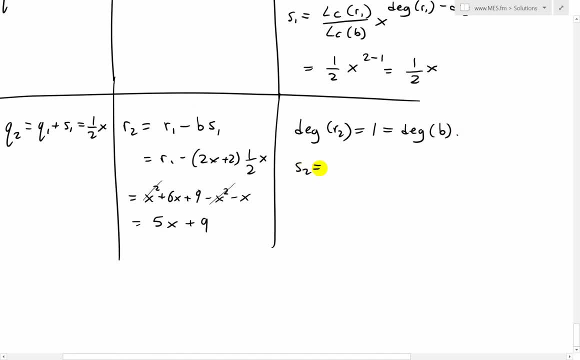 so thus we do a new S value. so S2 is going to be equal to the leading coefficient. yeah, so the leading coefficient of this is 5, divided by the leading coefficient of B is always going to be 2, and then we have now X. now the degree of R1, I mean R2- is 1, minus the degree of this one is 1, so we get 5 over 2X is 0, or just equals to 5 over 2, so that's what our S2 value is. 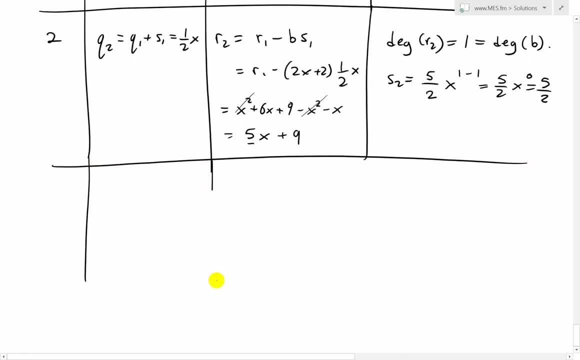 so that's what we have when we move on. So we move over here, expand this out. we get the third one here, or I'll put it over here: 3Q3 equals to- well, it's always going to be Q2 plus our S2, which equals to 1 half X plus S2 is 5 over 2, and then we just add that over here. so R3 equals to R2 minus BS2, which equals to, again, R2 minus now we have 2X. 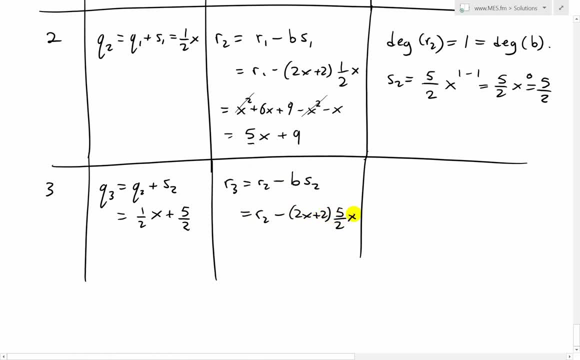 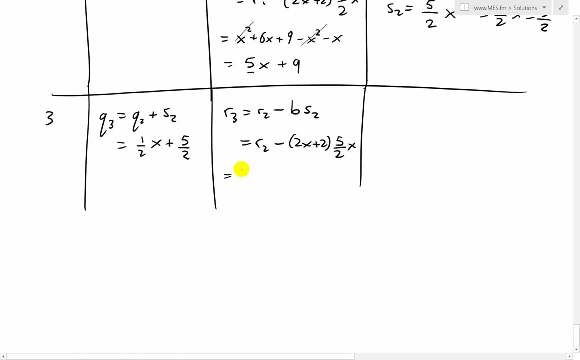 plus 2, and then we have this 5 over 2X over there. that's the S2 value. and then what we do? this R2 is just equal to 5X plus 9, multiply this out the 2s- cancel. we get minus 5X. so again, so we can cancel these out like that, then we have this minus 2s, cancel there, so we have minus 5,. yeah, this is an X. yeah, for that there's an extra X there. 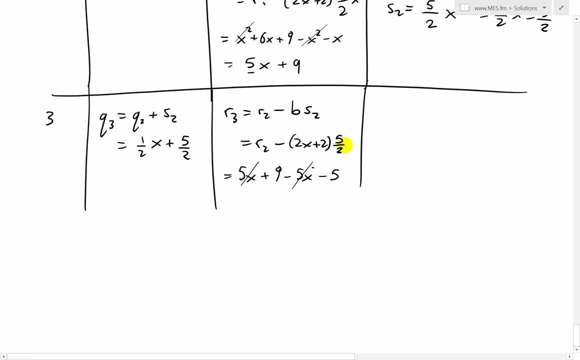 yeah, so mistake there. So we remove that X over there. yeah, so 5 over 2, there's still 5X there and this one negative 2 times 5 over 2, the 2s cancel negative 5.. 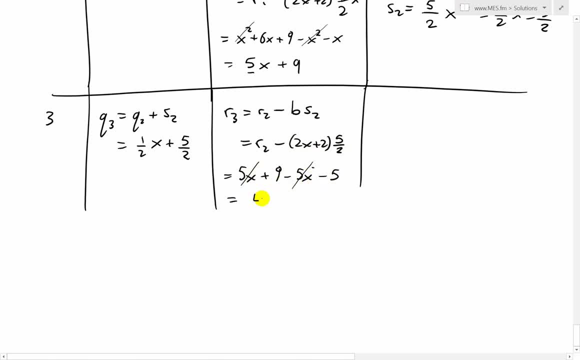 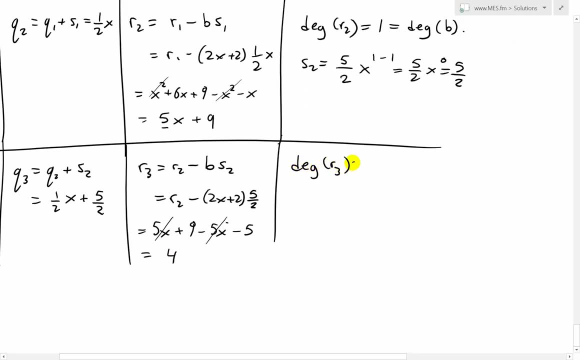 So this cancels. now what we're left with is 9 minus 5 is equal to 4, and that is our remainder. so now the question is: the degree of R3 equals to, well, 0,, that's just 4,. so that's equals to, and this is less than 1, which is the degree of B. 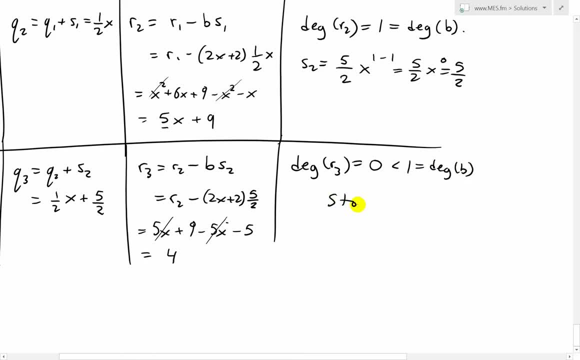 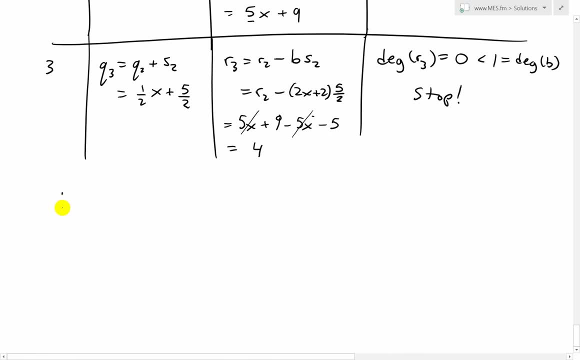 So what we do now is: well, we stop, And that is our remainder. so R3 is the remainder, and then what we have is thus: we have two values: Q3 equals to 1 half X plus 5 over 2, and R3 equals to 4, is the remainder. 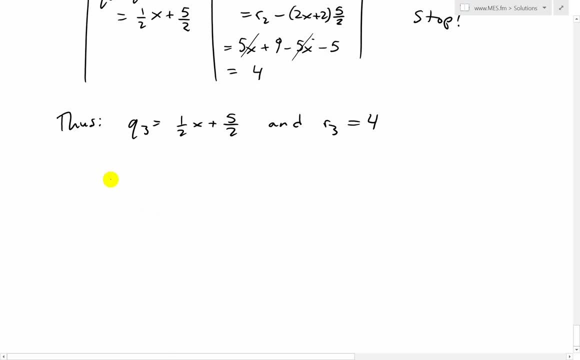 Yeah, and thus what we have is the overall one, A over B, yeah, which equals to our X squared plus 6X plus 9.. Over, like this, over the B2X plus 2, and long division, this just equals to now our Q3, which is 1 half X plus 5 over 2, and then plus the remainder over there, which is just the 4 divided by 2X plus 2 as a fraction. 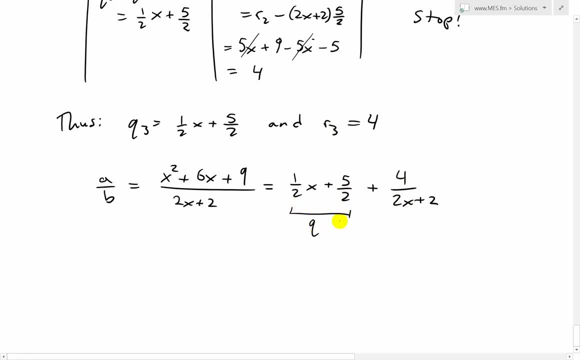 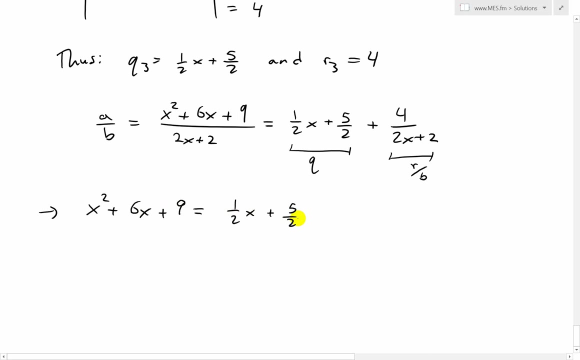 Yeah, so that's our A over B, this is our Q and this is our R over B. In other words, put that in the Euclidean division In one, we have X squared plus 6X plus 9 equals to 1 half X plus 5 over 2, move this over, that's our Q, times it by 2X plus 2, and then multiply it like that plus 4 as a remainder. 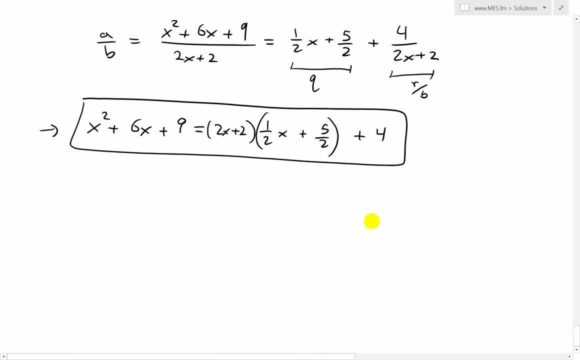 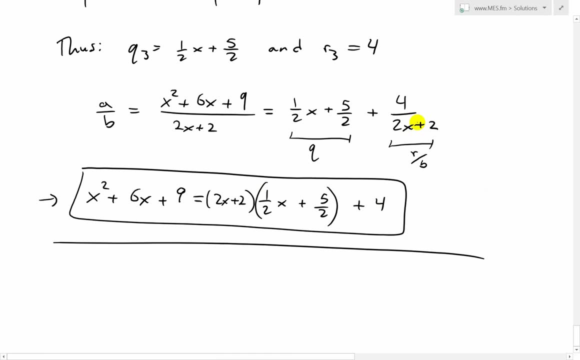 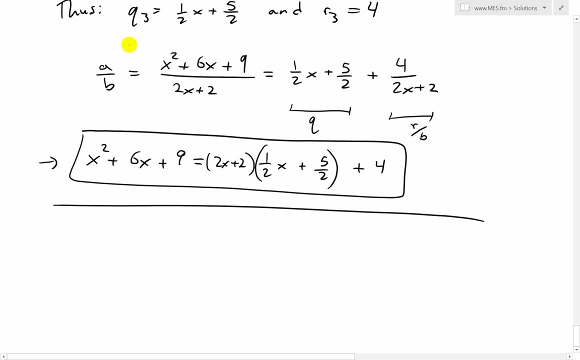 So there is our Euclidean division, like that, For example. it is exactly the same thing. you just divide it out or multiply it out, like that, and then you get it in this form like that, Absolutely amazing stuff like that. Move this down and circle this answer. 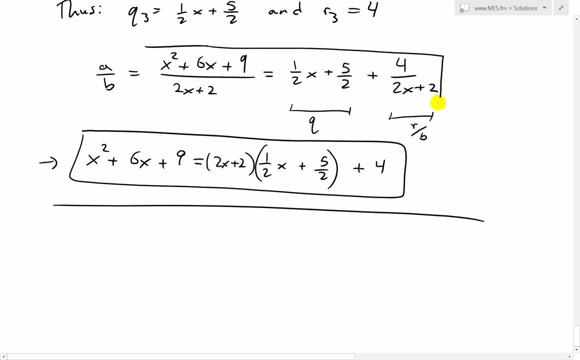 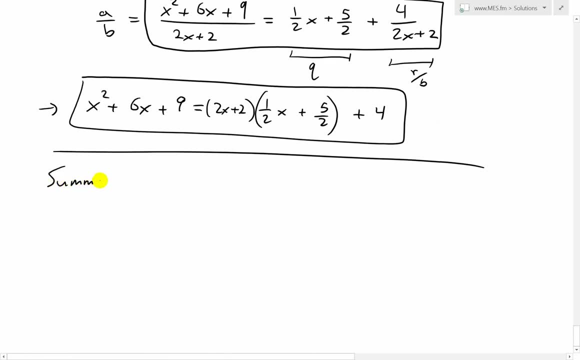 And it's exactly the same answer we did using the long division, which is: this is actually the long division method, proof for it as well. And now, just to summarize all this, a summary. just wanted to do an example in this video just to illustrate it all better. 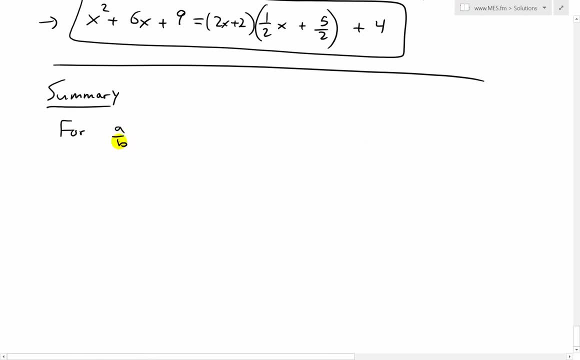 Summary for A over B division. or you could write it as A: A slash B or A divided by B, or we have it as this method or this long division: B over A, and A and B are basically univariant or single variable. 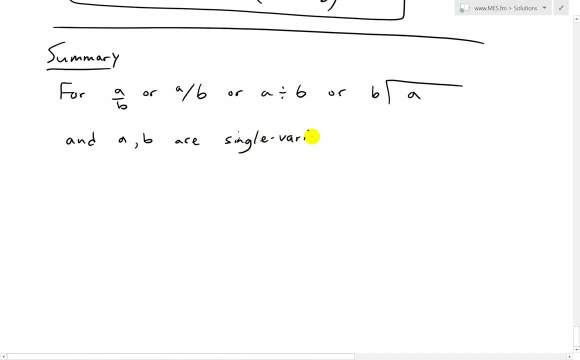 I'll write single variable, or yeah, this is basically univariant. You could write it as that, or univariate polynomials, polynomials, and then with B is not equal to 0, so you can have that. Then what we have is a Euclidean division: A equals to BQ plus R, like this with degree of U. 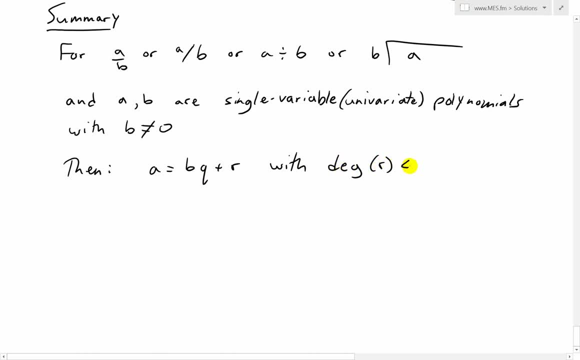 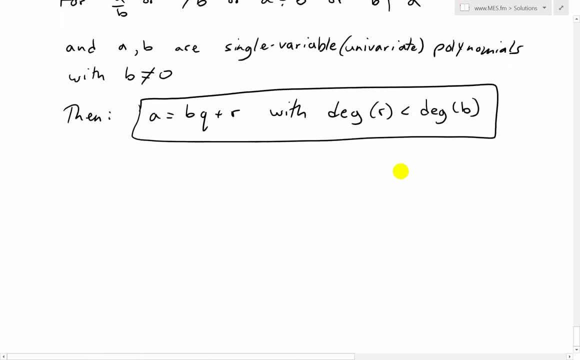 Here, degree of R is less than the degree of B, so we're going to have eventually one like that over there, And if degree of R is, it's not degree of R, and if R equals to 0, yeah. so if R is equal to 0, assume a degree of 0.. 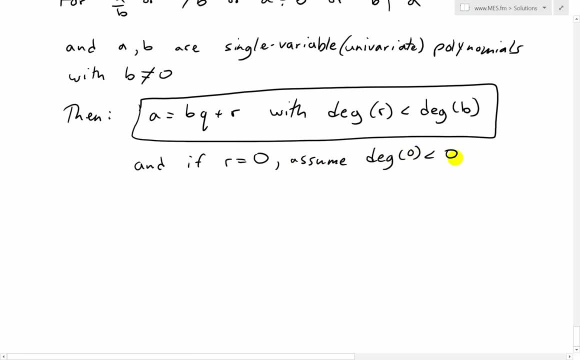 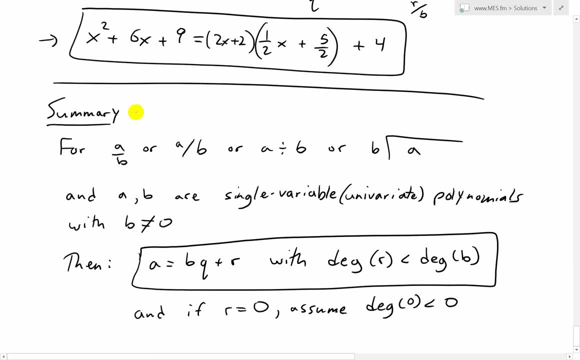 And that is, yeah, assume it's negative, and that's for algorithm purposes. if we have the case where B is degree of B is 0.. And yeah, this is summary of Euclidean division for polynomials. Euclidean division, just put it all, completeness sake. 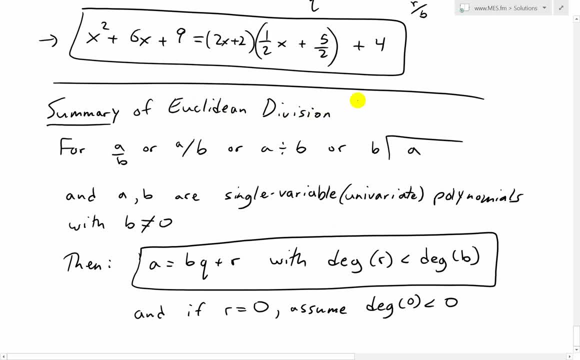 So if you've seen all this whole video, or a couple more minutes, it's not going to do too much. So Euclidean division for polynomials like that, And yeah, that's it. That is all for today. Keep going further like this: 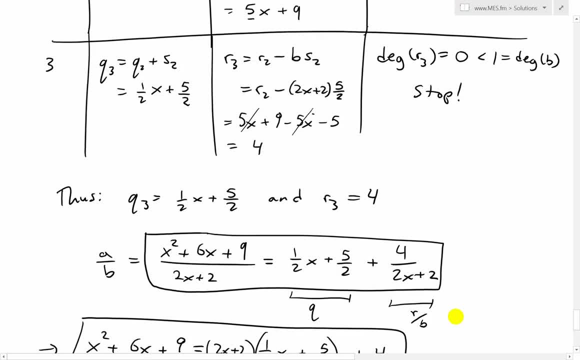 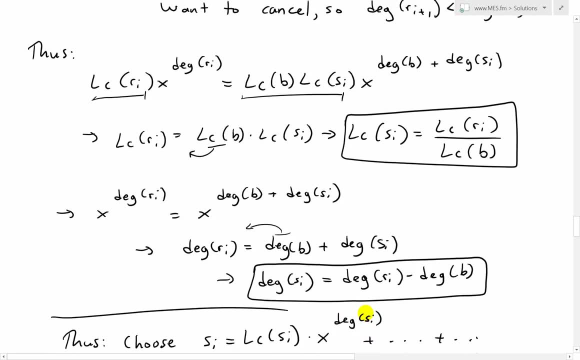 Yeah, so that's all for today. I hope you follow along. It's a pretty extensive video but if you've watched the whole thing, you're pretty much an expert in Euclidean division, Because I like to do it, even if it's long, as long as you know it full well and it'll help you later in other math and division and algebra and so on.